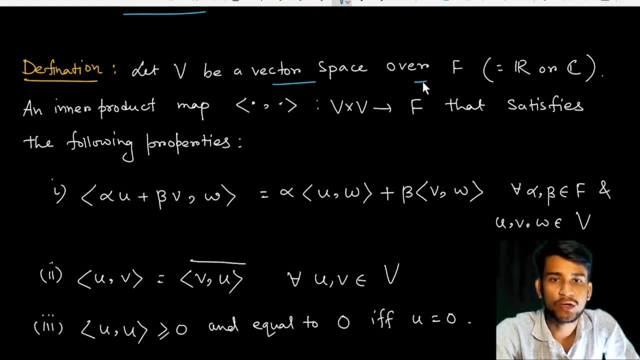 product. So let V be a vector space over the field F, that is, R or C, and inner product is a map, that is, this is the defined two dot and dot. just this is a notation. So this is a function from V cross V to F such that it satisfies the following properties: The properties number one: 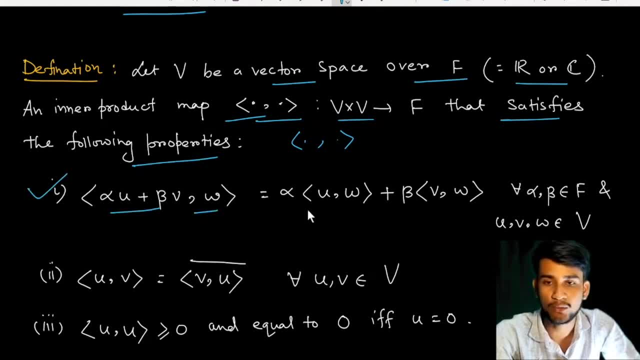 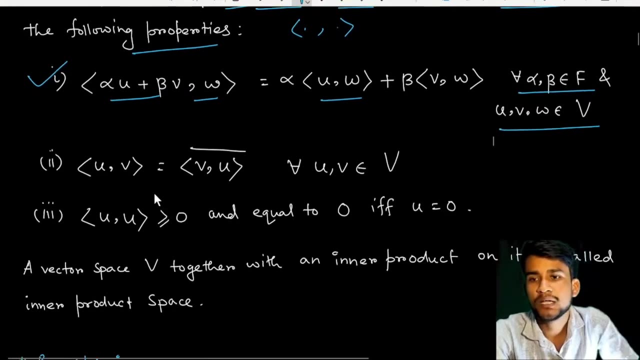 is alpha of U plus beta of V in comma W. this is equal to alpha into U W plus beta V W, where alpha beta belongs to the field F and U V W belongs to the vector space V. So next, the second property is U V equal to V U complement. So this is, since this is a general vector, that is, the vector may. 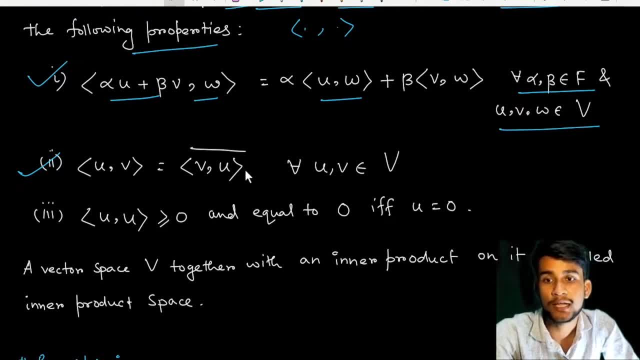 be belongs to the complex number C. So that is why we take here the complex conjugate, So U, V, this is equal to V, U complex conjugate. and number three is U, U greater equal to 0 and equal to 0, even only U equal to 0.. 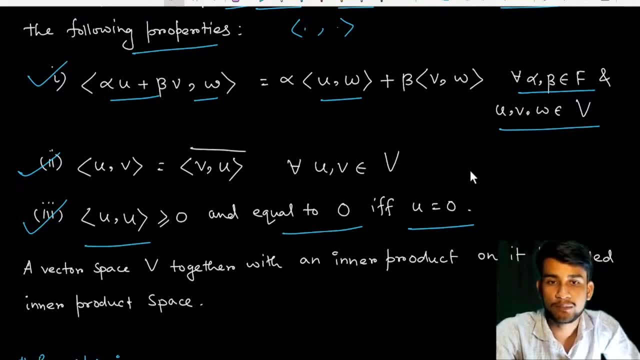 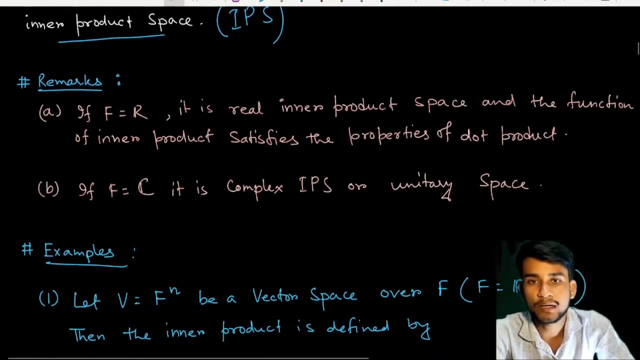 So if a function V cross V to F satisfies these following three properties, then a vector space V, together with this inner product on it is called the inner product space or IPS, inner product space. So now comes to an important remark. the remark is one: if F equal to R, then the real inner 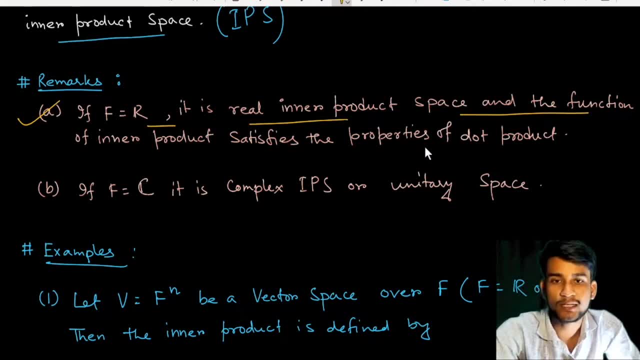 product space and the function of inner product satisfies the following dot product, So that the field is R, then we mean by the we mean the dot product same as the inner product, and if F equal to C, then it is complex inner product space or unitary space. So let us take the examples So. 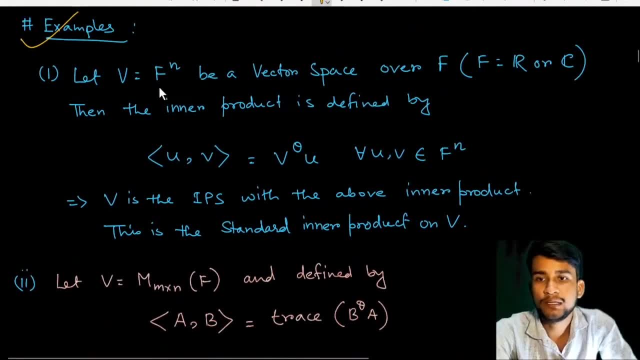 the example. one is what? let V equal to F, power n, where F to the power n, that is, F, tuple n, tuple of the space, be a vector space over the field F, F equal to R or C, then the inner product is defined by U. b equal to V, dagger into U. this is the complex. So that means we know, already know. 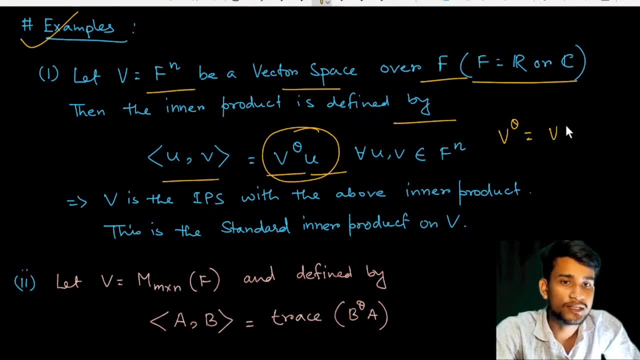 that V theta equal to V theta, V t then transpose, So the V theta, V transpose, and then the complex conjugate. So this is the defined and in real, this is simply V transpose. This is simply V transpose U. So for all U b belongs to n tuple of the field. 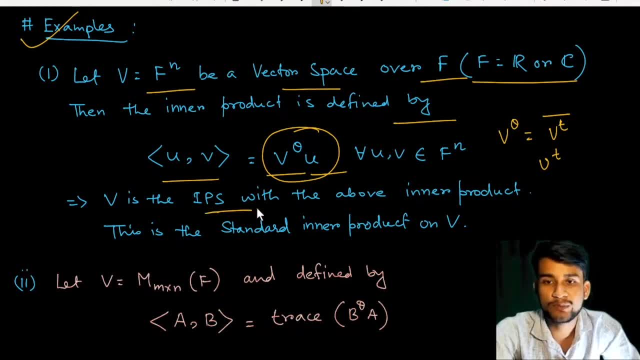 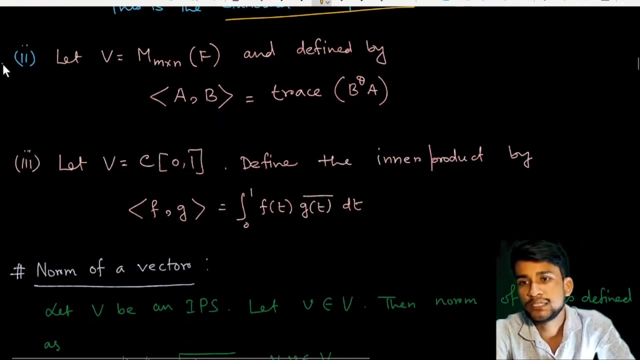 F. So then V is an inner product space with the above inner product. This is the standard inner product on V. So this is the example of standard inner product on V. The space is where the space is. this field, Now number 2, is in the matrix field. the inner product is defined by: 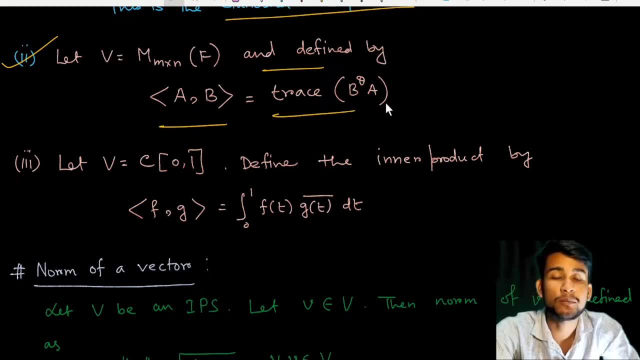 A into B, inner product of A, B. This is equal to trace of bit theta A And this is the general. in general, in the space, complex space, In the real space, this is equal to trace of B. transpose A simply, And this is the matrix inner product. And for the case of function, let us V equal to. 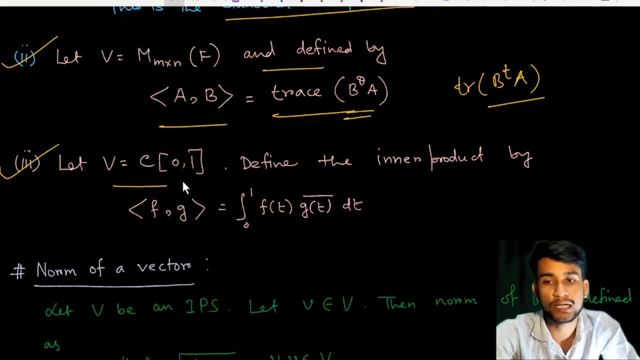 C 0. that is, the difference able functions over the continuous difference able functions or removed function over the interval 0- 1.. Define the inner product by inner product of F- G. This is equal to integration 0 to F T into G, T, bar into D T. This is the complex conjugate of the 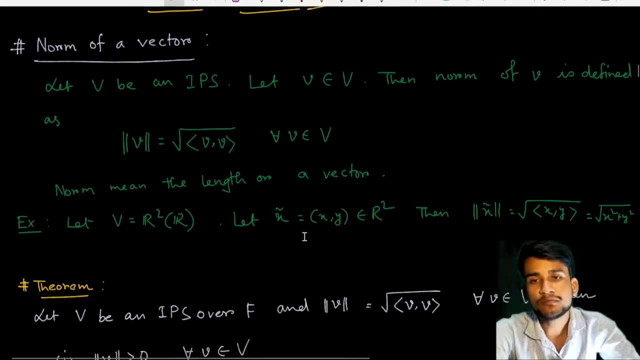 function G, T. So now this is. these are the examples of the inner product. Now it comes to an important definition, which is the norm of a vector. So what is the norm of a vector? Let V be an inner. 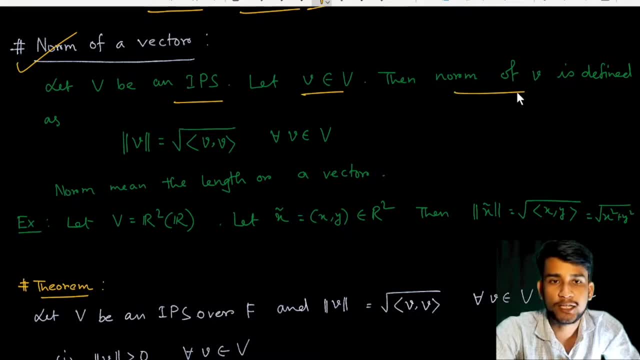 product space. Let V belongs to B, Then the norm of the vector B is defined by norm of B. This is equal to root under inner product of V and B, for all V belongs to capital V, So norm means the length of the vector, length or of a vector. 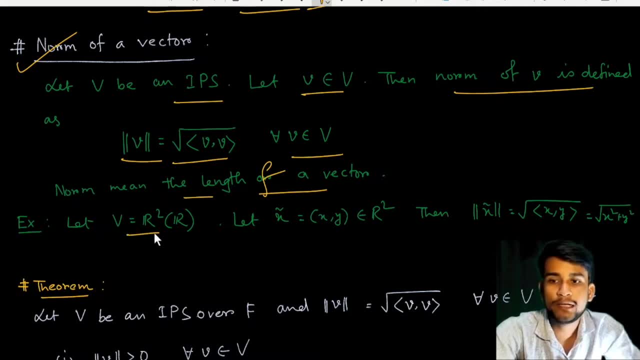 So length of a vector. For example, let V equal to R, 2 is the vector space over the field R. Let the vector X is equal to X, Y belongs to R 2. Then norm of the vector X is equal to a root under of X into. 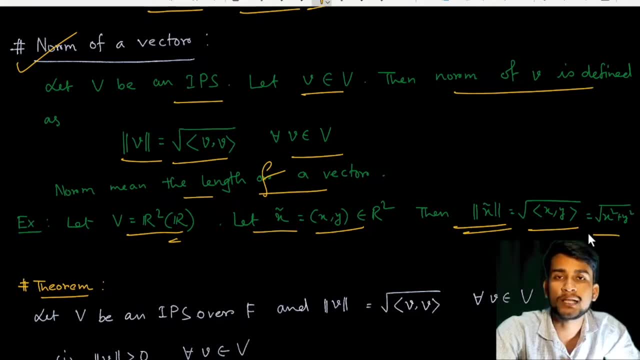 Y. So this is equal to simply root under X square plus Y square. We all know the length of the vector formula, So this is simply the formula of length of a vector. Now let us come to an theorem. So this is the formula. 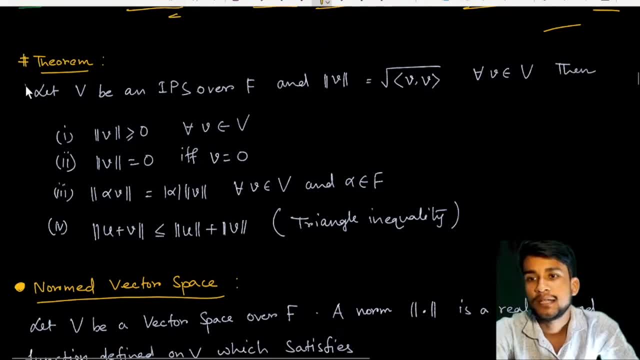 Now let us come to an theorem. The theorem is: let V be an inner product space. Let just a minute, Let V be an inner product space over F and norm B, equal to root under inner product of V and B. for all V belongs to B, Then number 1 is norm B is greater than 0. for all V belongs to B, Number 2: 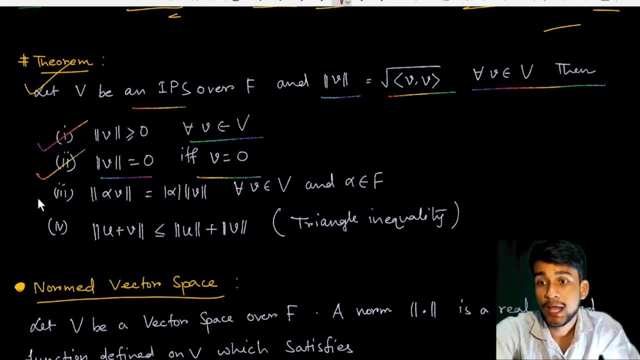 is: norm B is equal to 0, even only B equal to 0, and norm of alpha B equal to mod alpha. norm B for all alpha belongs to B, So this is equal to 0.. Now let us come to another theorem. Now let us come to. 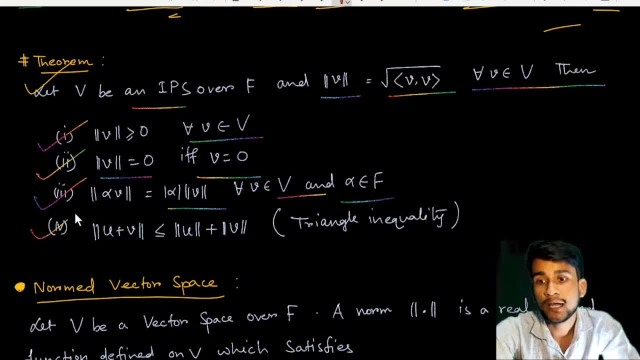 to b and the alpha is the member of a field and number 4 is norm of u plus b less equal to norm u plus norm b. this is the triangle inequality. you all know that. So inner product space over f, then this is the. this is the theorem that is. I think so. this is the theorem that is. this is the inner. 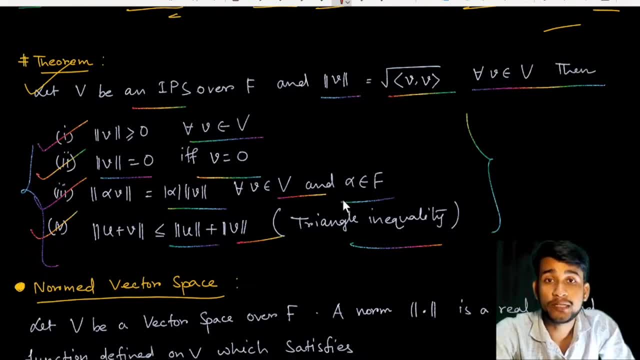 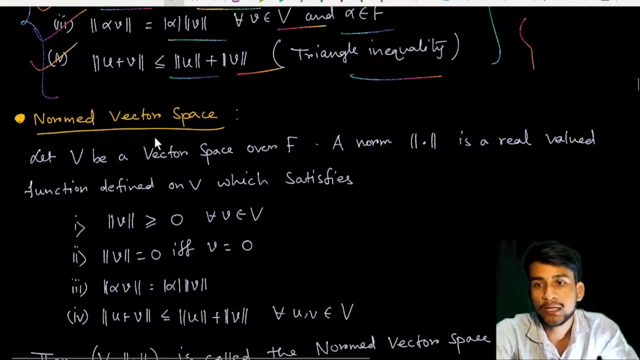 product space and sorry, this is the theorem in norm space after defined norm, then it comes to this theorem. that means what that means: an inner product space is a norm space also. let us comes to that point. So norm vector space- this is the norm defined norm vector space. what is the norm? 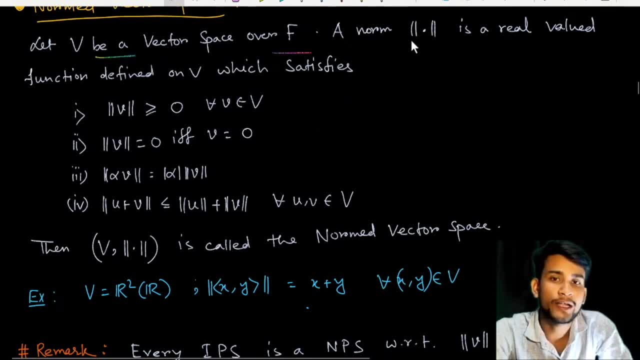 vector space. let v be a vector over f and a norm is defined. is a real valued function defined on this which satisfies this. this four above properties, then v is norm, is called the norm vector space. So these four properties are very important. So these four properties are very important. So these four properties are very. 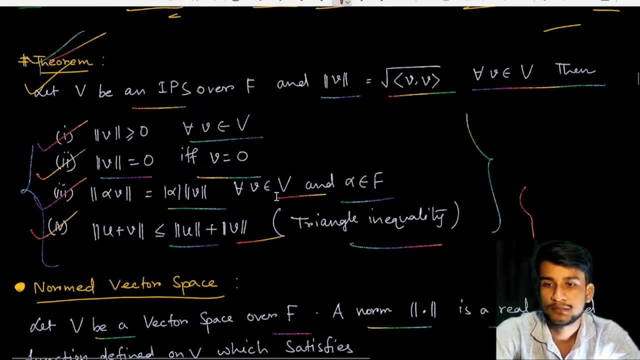 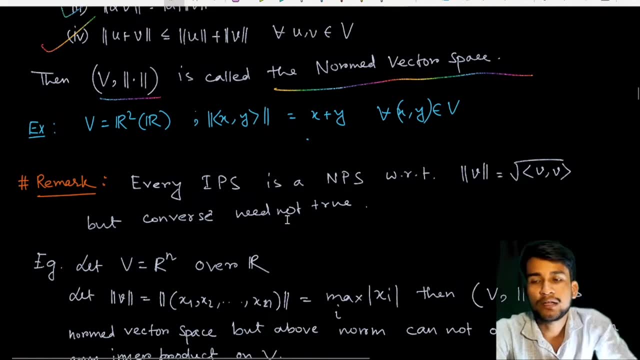 important for the case of norm of a vector. satisfies for norm of a vector satisfies norm. satisfies this four properties. this is the theorem. and, for example, let v equal to r to over r, then norm of x- y: this is equal to x plus y. this is a simple example of a norm of a vector space. 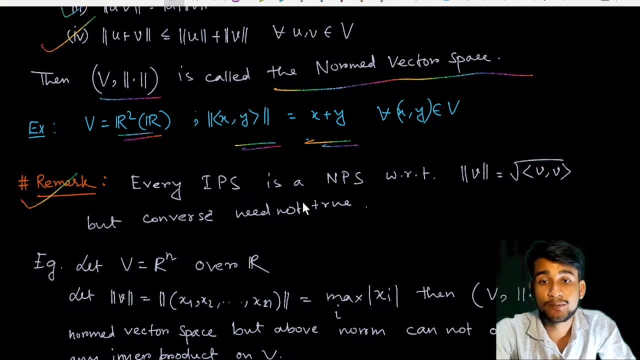 Now, an important remark is: every inner product space, every inner product space is an norm vector space. norm vector space, that means inner product space implies what ips implies- nvs, just a minute- and inner product space. inner product space implies a norm vector space. So let us comes to an example: let v equal to rn over. 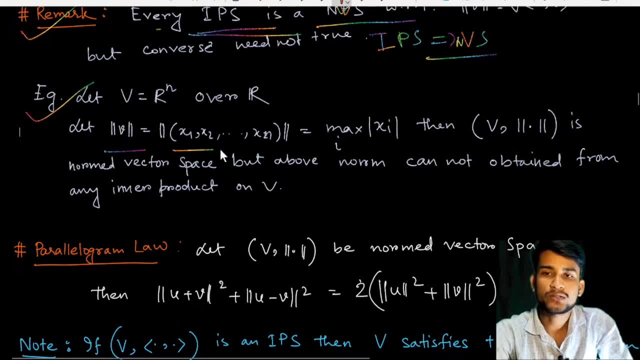 r, then norm v, equal to norm of x1, x2, dot, dot extension. this is equal to the define defined by max of mod i, then v, and a norm with this norm is norm vector space. but the above norm cannot obtain from any inner product space, that is. this is the example, that is, ips, implies nvs, that is, inner product space. 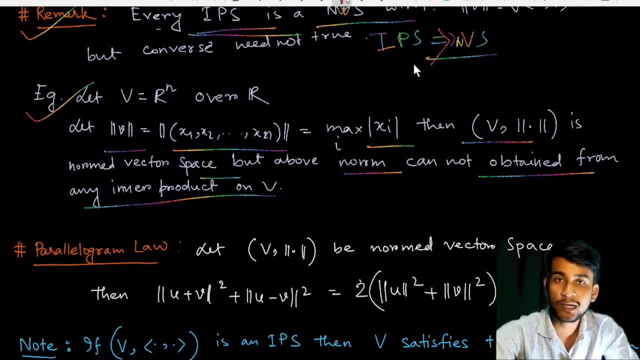 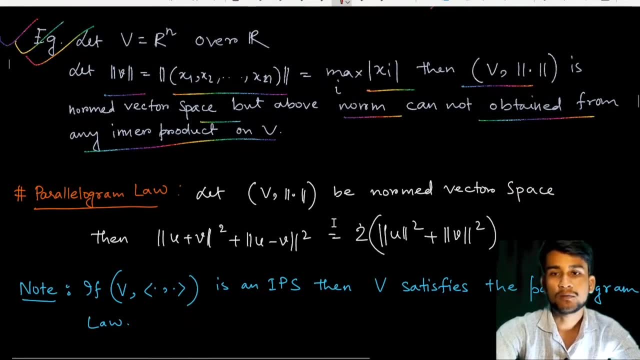 implies inner product space, means norm vector space. but norm vector space means does not imply the inner product space. So let us come to an example. let us come to an example. let us come to an product space. This is the example for that. okay, Now it comes to parallelogram law. What? 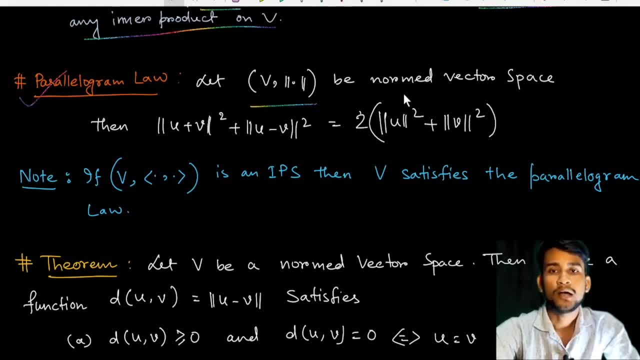 is parallelogram law. Let v norm with a norm where norm vector space, then norm of u plus v whole square. this is plus norm of u minus v whole square. this is equal to 2 into norm of u square plus norm of v square. Here an important note is if v norm v with the inner product is an 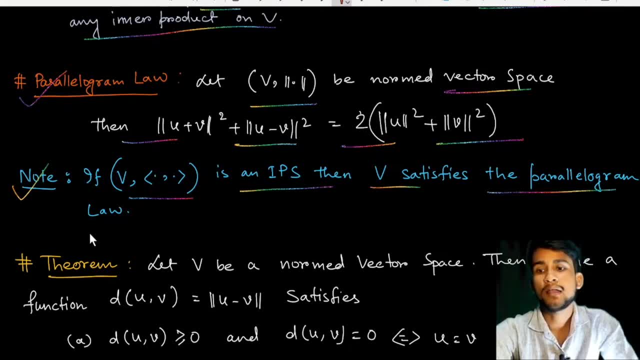 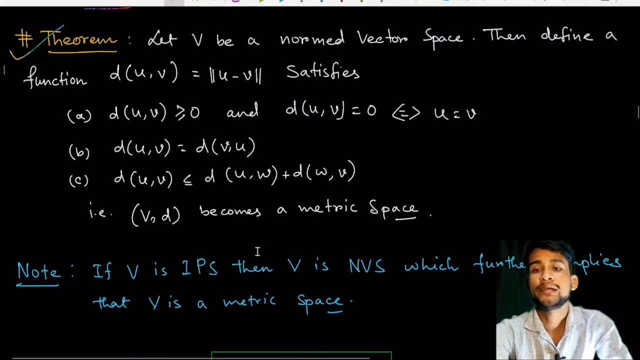 inner product space with, then v satisfies the parallelogram law. okay, That means, if v is an inner product, v with an inner product is an inner product space, then it satisfies the parallelogram law. okay, So let us come to a theorem. The theorem: let v be a norm vector. 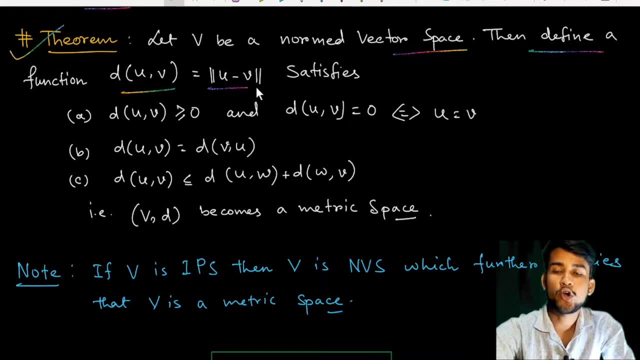 space. then define d of u v. this is equal to norm of u minus v. satisfies d of u v greater equal to 0 and d of u v equal to 0, if only u equal to b, Number b is d of u. 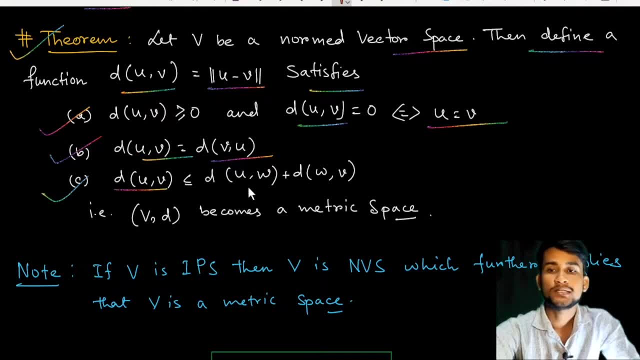 b equal to d of v. number c is d of u v. this is equal to d of u w and d of w v. That is, if we take any vector in between u and v, then this satisfies the linearity, or less equal to. 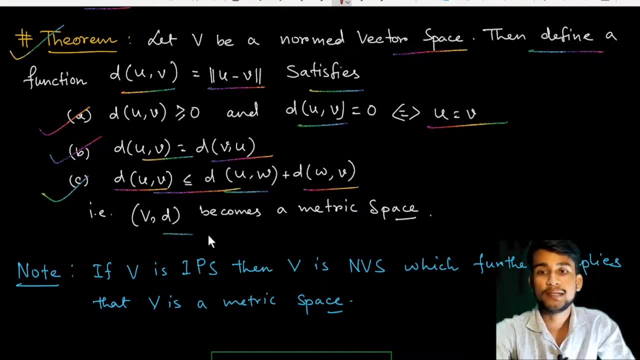 type or triangle inequality properties. okay, So this v? d becomes an matrix space. This is the three properties, main properties of matrix. we all know that. Therefore, a norm vector space is also a matrix space. That means an inner product space. this implies norm vector space. 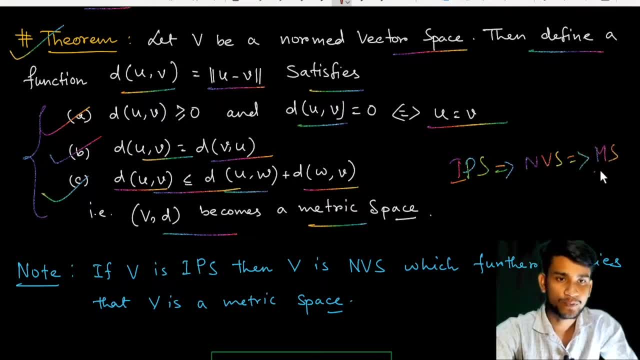 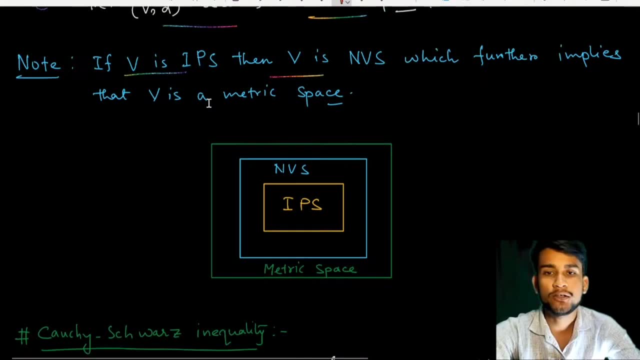 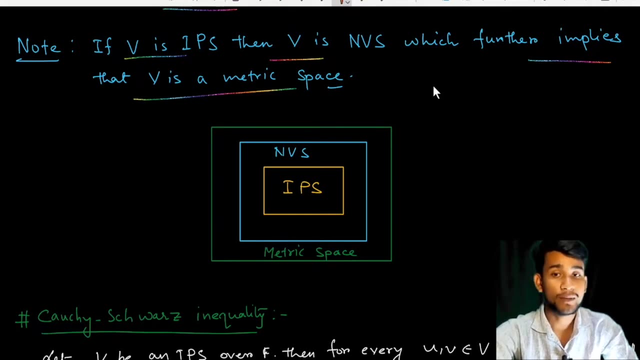 this implies also a matrix space. okay, That means we note the note is: if v is an inner product space, then v is an norm vector space, which is further implies the v is an matrix space. So this is very important statement. okay, We can remind this statement for the. 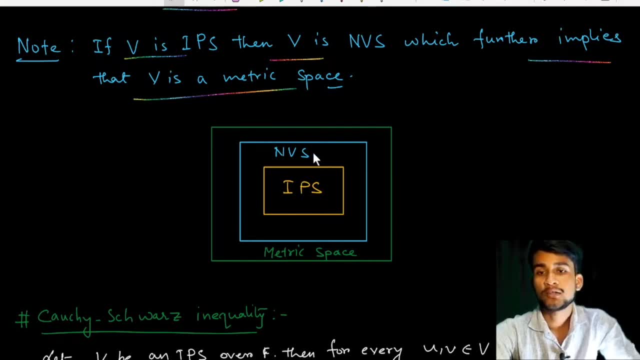 further and for future response. okay, So inner product space is the inner. that is inner product space, then that means see from this picture, remind this picture. inner product space implies norm, vector space, implies matrix space, but matrix space does not. 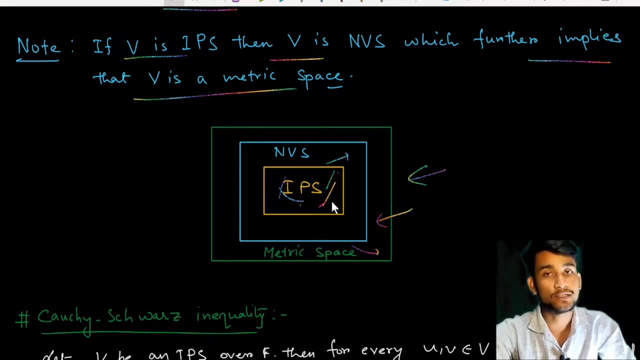 implies norm vector space or matrix space. does not implies inner product space. okay, We also take the examples above. that is for the case of n. vs does not implies ips. okay, So this, we can take the example. another examples also. okay, Now let us come. 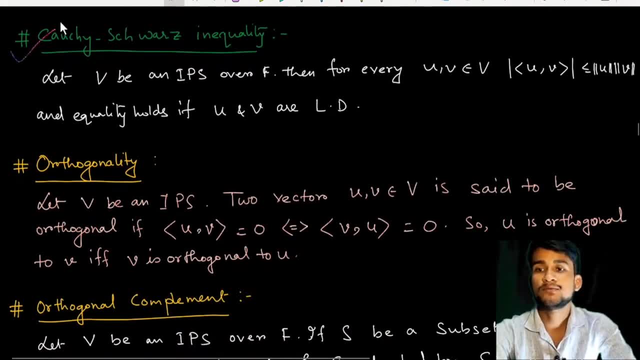 to an important inequality, which is Cauchy-Schwarz inequality- This is very important. inequality and inner product space over f. then for the following: for every uv belongs to b mod of the inner product, u and v. this is less equal to norm of u into norm of b. okay, And equality. 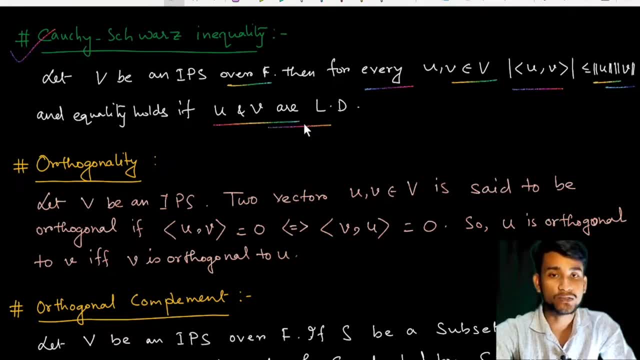 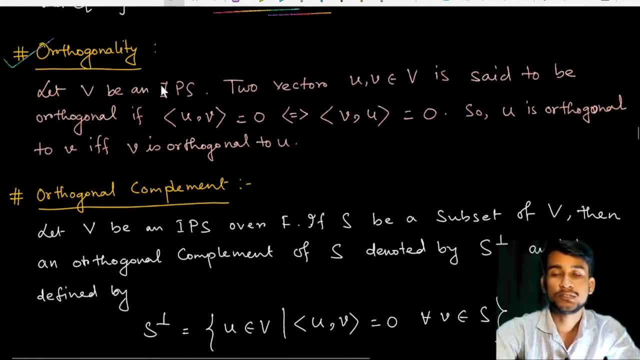 holds, even only if uv are linearly dependent. okay, So this is very important. inequality: okay. Now let us come to the, an important concept, which is orthogonality. This concept is also very important, So let v be an inner product space, then two vectors: u and b. 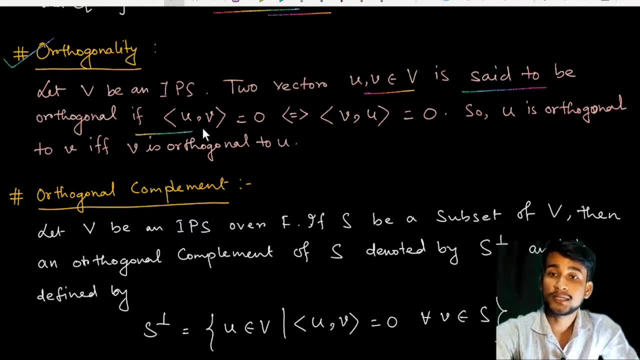 is said to be orthogonal if, and only if, their dot product, that is the inner product of u and v, is equal to 0. And we also know that in simple linear algebra, if the dot product of any two vectors is 0, then we say that the two vectors are orthogonal to themselves. okay, So the similar 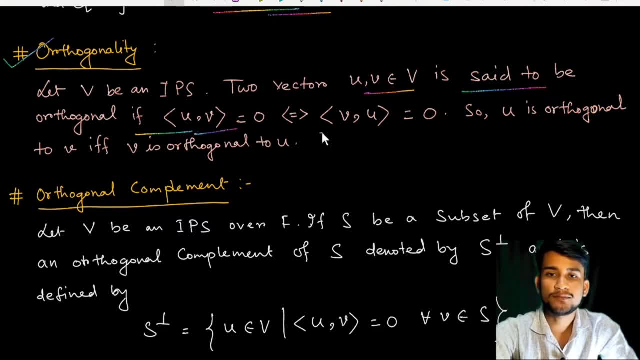 concept in the inner product space also. okay. So this implies v equal to 0.. So u is orthogonal to v. this is if, and only if, v is orthogonal to u. that means the vectors in the simple vector space. orthogonal means what The vector is perpendicular to another vector and 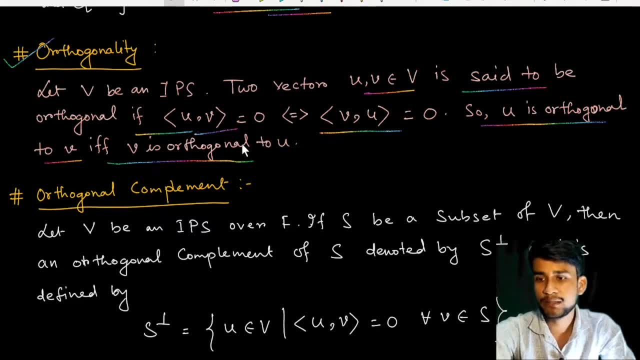 the other vector is also perpendicular to the rest of vectors. So there is the same concept. okay, In, just just we change the space. okay, This is not the vector space, this is an inner product space. Now let us come to the another definition: orthogonal complement. okay, Let v be. 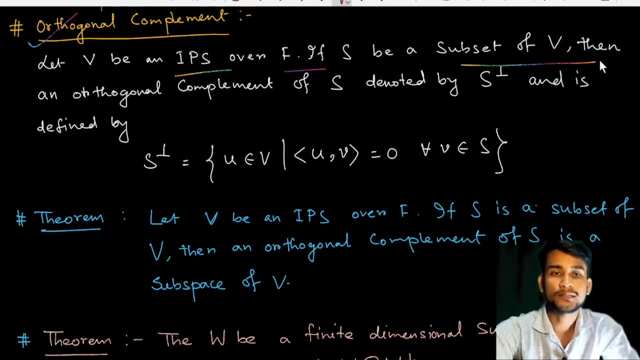 an inner product space over f. if s be the subset of v, then an orthogonal complement of s is perpendicular, okay, And is defined by s: perpendicular. this is equal to: u belongs to v, such that the inner product of u and v equal to 0 for all, v belongs to s. then we say that: 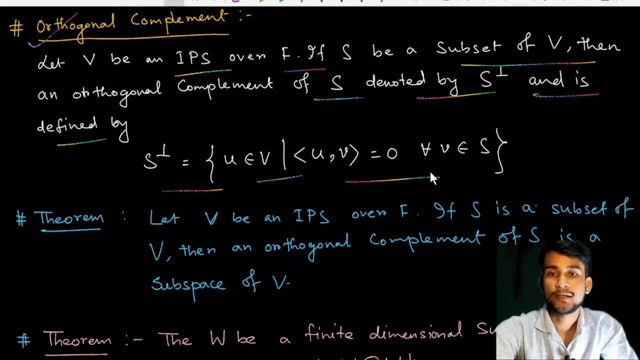 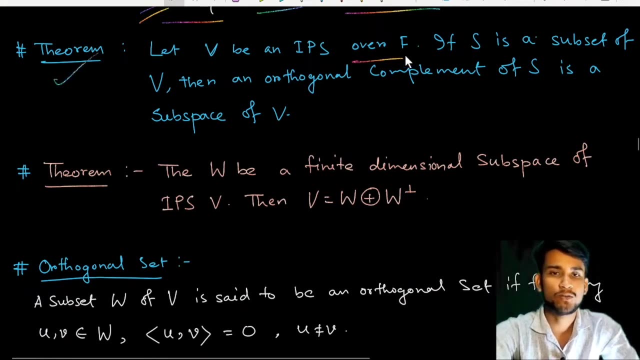 the set is called a orthogonal complement of the. this s set is the vectors. contains that vectors which are orthogonal complement with the another vector? okay, And this is the definition. Now let us come to an theorem. The theorem is: let v be an inner product space over f if s is a subset. 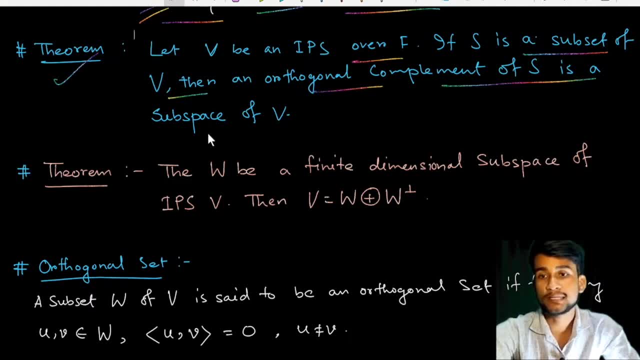 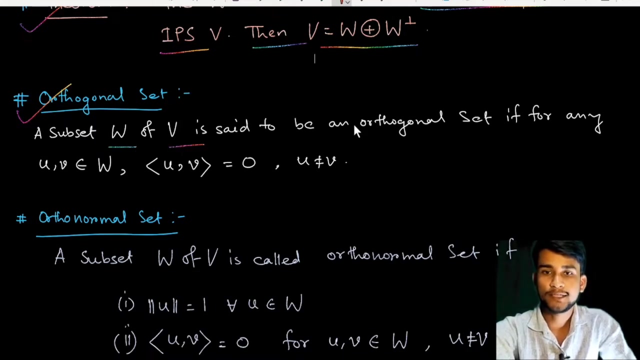 of b, then an orthogonal complement of s is a subspace of a, which is an result type. you can say: And the next theorem is: let w be a finite dimensional vector space of an inner product space, v, then v equal to w and plus. this is what is orthogonal set. okay, A subset w of b is said to. 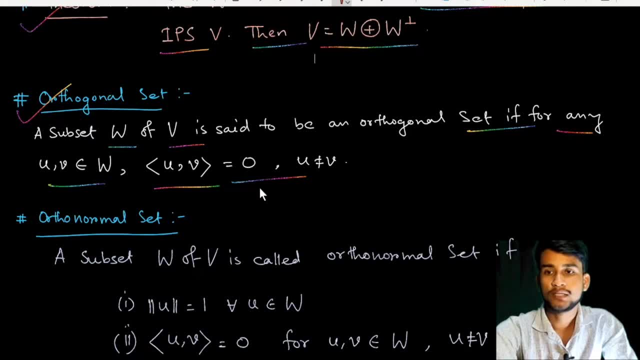 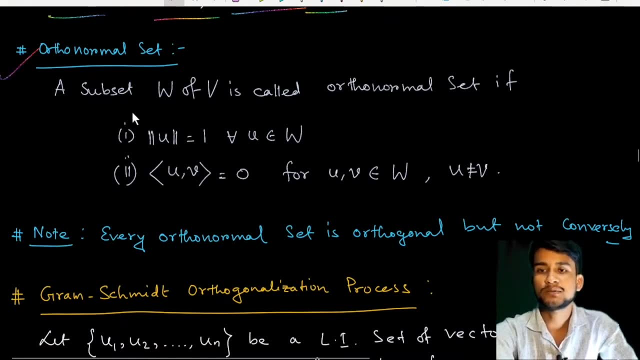 be an orthogonal set. if s is a subset of u and v equal to v, then the set is called an orthogonal set where u is not equal to v. Now it comes to orthonormal set. what is orthonormal set? A subset? 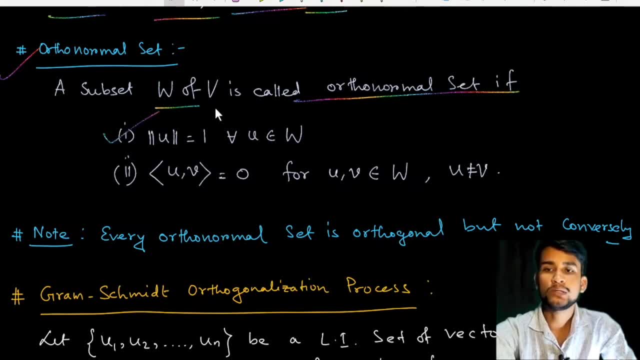 w of b is said to be orthonormal set. if norm of u equal to 1, for all u belongs to w and u v. norm of u? v that is the dot product of u, v and v, this is equal to 0, for all u v belongs to. 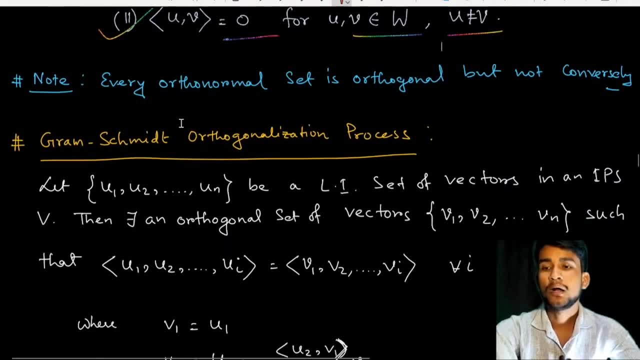 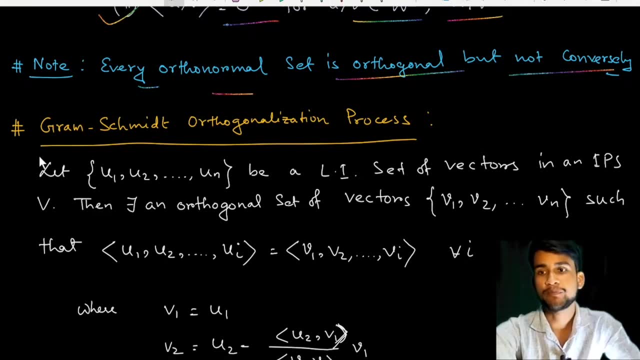 w for u not equal to v. okay, Now a note. important note is: every orthogonal set is an orthonormal set. it is orthogonal set but not conversely. okay Now, Gram-Smith's process. just say the process, we do not go to the details of this process. okay, because if we go to discuss, 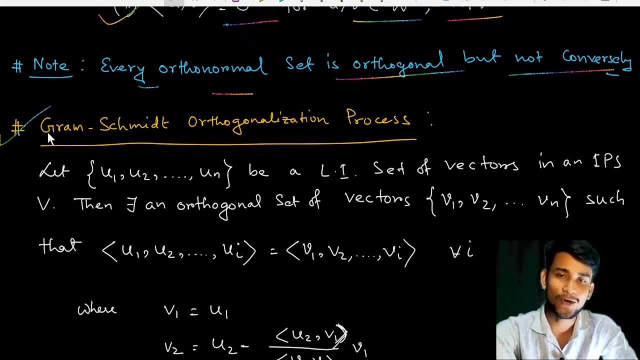 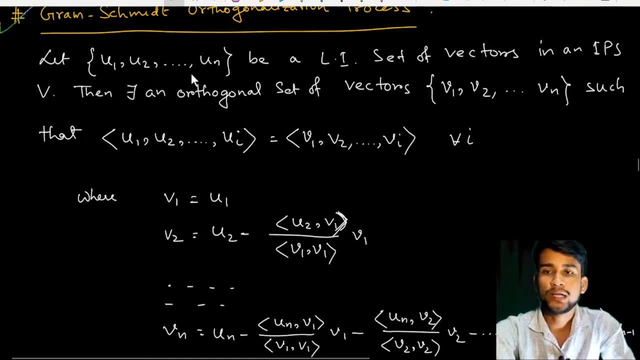 this process. then it said it: this theorem takes a long process and a long time, okay, So that is why we skip the complete process. we just write it, okay. So let u n? u 1, u 2, u n be the. 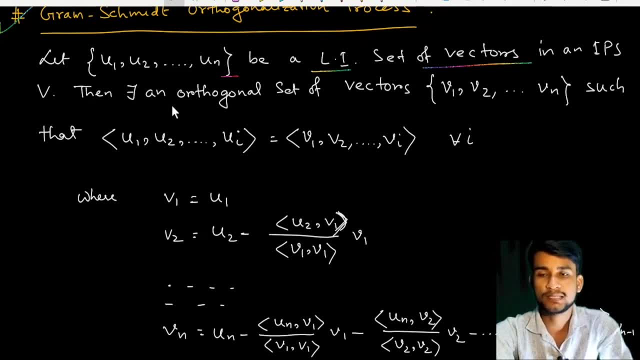 linear, independent set of vectors in an inner product space. then there exists a orthogonal set and if you want, then I also make a separate video for Gram-Smith process. okay, So comment me if you have. if you need this, okay. Complete set of vectors v 1,, v 2, v n, such that u v. 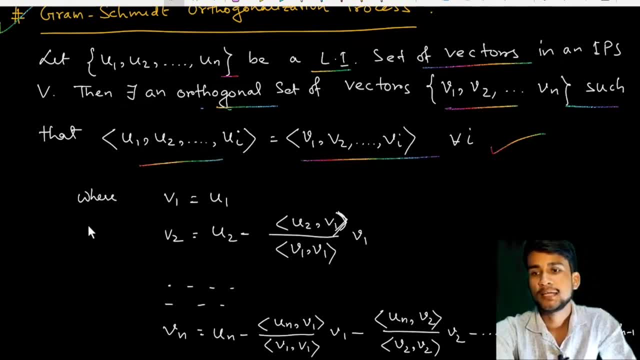 u 1,, u 2, u i. this is equal to v 1, v 2, v i for all i, where that means we have given a set of vectors and we have to construct a orthogonal set of vectors or orthonormal set of vectors. 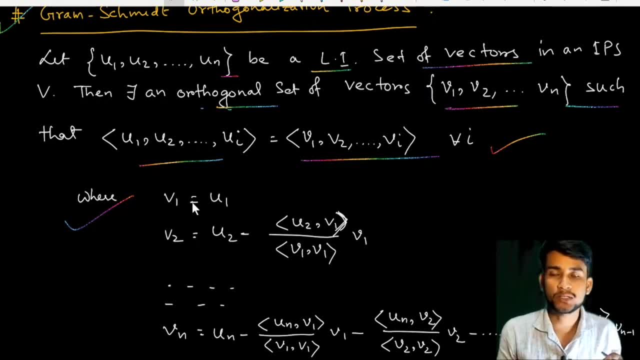 Gram-Smith process actually doing what doing Gram-Smith process is actually do: to construct the set of vectors to a orthogonal or orthonormal set of vectors. okay, So this is the work for the Gram-Smith process there are. this is the. 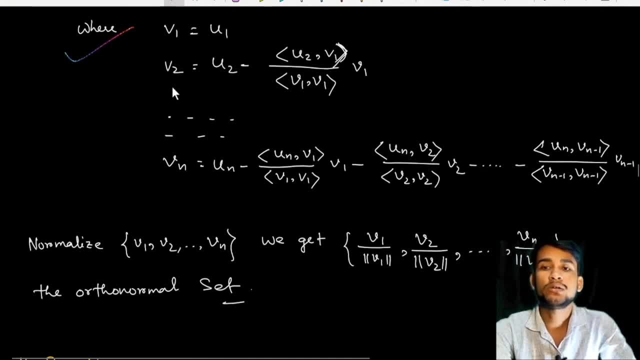 importance of the Gram-Smith process. okay, So v 2 equal to u t minus this one. your dot product of u 2, v 1 by v 1, v 1, inner product into v 1 and the general formula. you just remind this line. 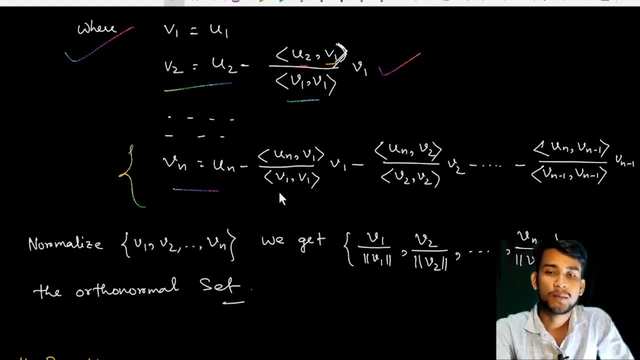 okay, So v n equal to u n minus u n v 1 by v 1, v 1 into v 1, and so on, and up to u n v n minus 1 by v n minus 1, v n minus 1 into v n minus 1,. 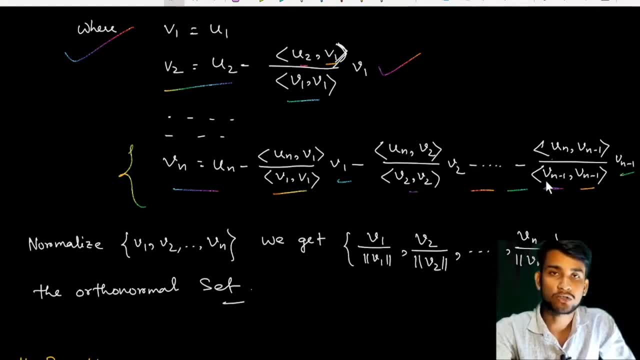 okay, So this is the general formula to construct the orthogonal vectors. okay, v 1,, v 2,, v n, And after norm, after we getting the orthogonal set of vectors, we just normalize the vectors to get an to get the set of orthonormal set of vectors. okay, So the orthonormal set of vectors. 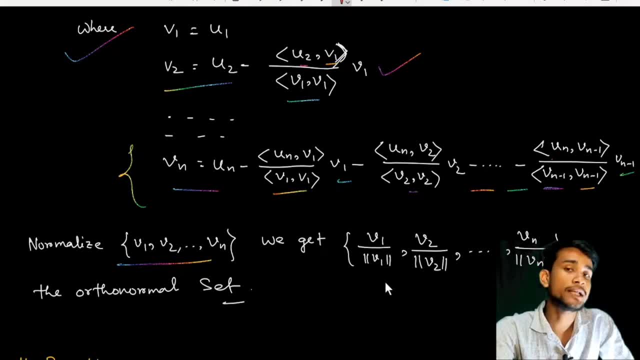 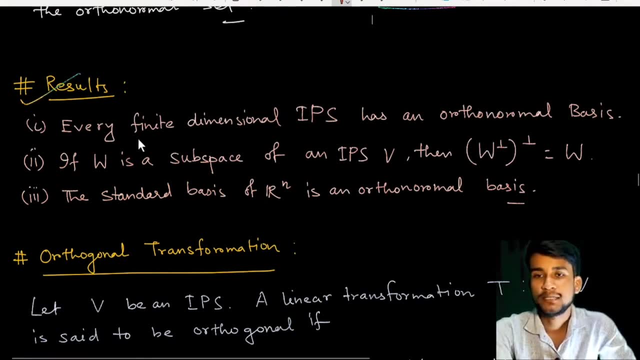 just we divide the vectors with their norm. okay, We get the orthonormal normal set of vectors. Now important result is: every finite dimensional inner product space has an orthonormal basis. this is an important theorem or result. if w is a subspace of an, 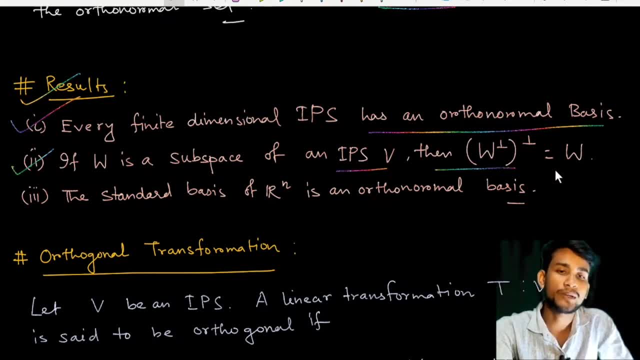 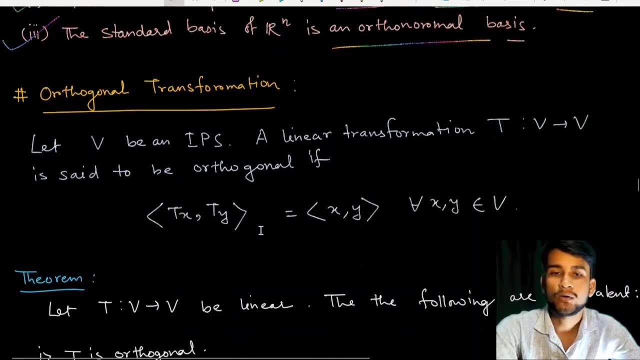 inner product space: v then w, perpendicular then perpendicular, this is equal to w, and the standard basis of R n is an orthonormal basis. And now it comes to an important part: the orthonormal transformation, or orthogonal transformation. this is a big part. 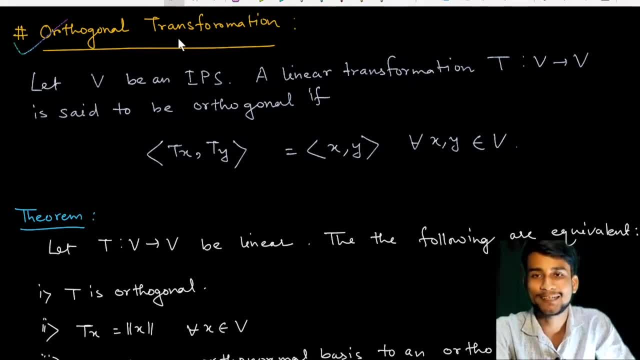 I just write one or two result and the basic criterion, and just this. since this is a small discussion, okay, because inner product space is a huge topic. okay, So we just here discuss a to the point, point to point. okay, So let v be an inner product space. 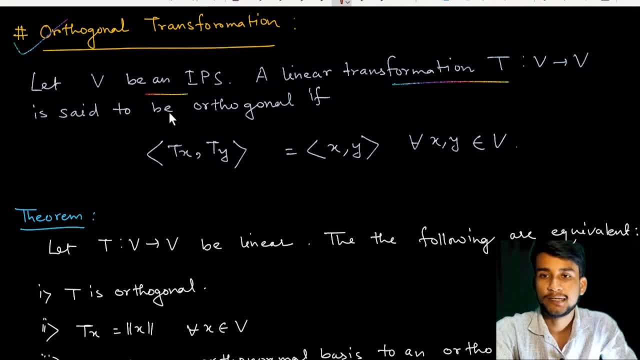 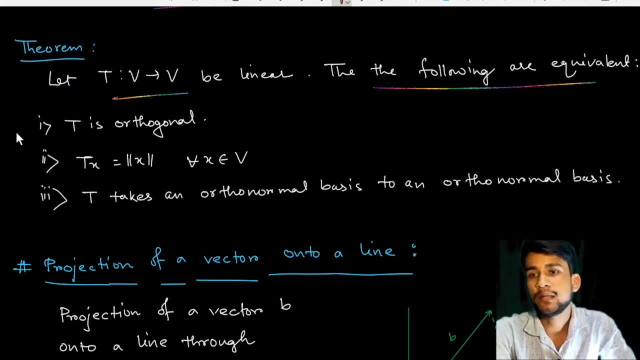 a linear transformation, t from v to b is said to be the orthogonal. if t x, t y, this is equal to x into y, for all x, y belongs to v. okay, Now let us comes to another theorem. let t from v to b be a linear. then the following are equivalent: t is orthogonal, t x equal to norm. 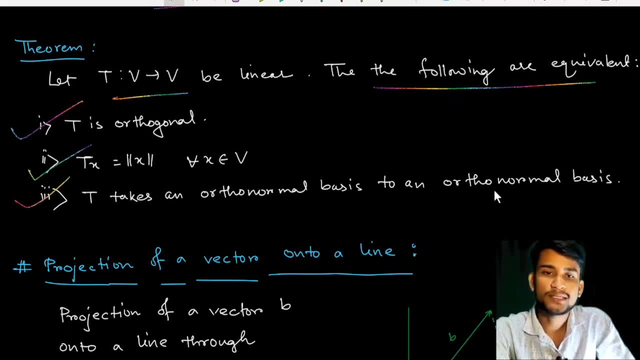 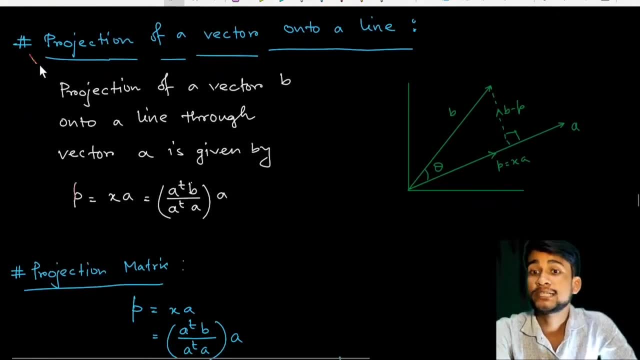 x for all. x belongs to v, t takes an orthonormal basis to an orthonormal basis. that means t is also 1, 1. you can say: okay. Now it comes to a very important concept, which is projection of. 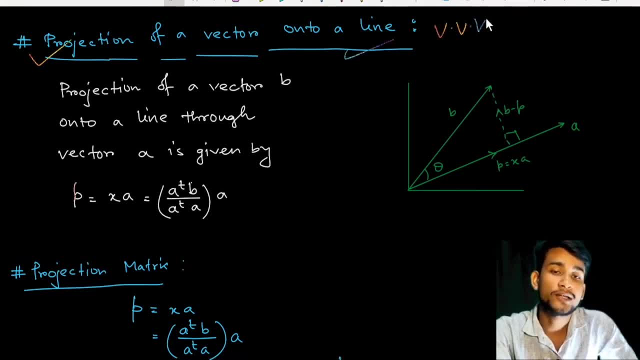 a vector onto a line? this is a very important question because based on this concept, questions comes in: CSR, net, also get, and TFR, NBHM, all types of, in all types of exam in any question paper. or you can say: if we, if we. 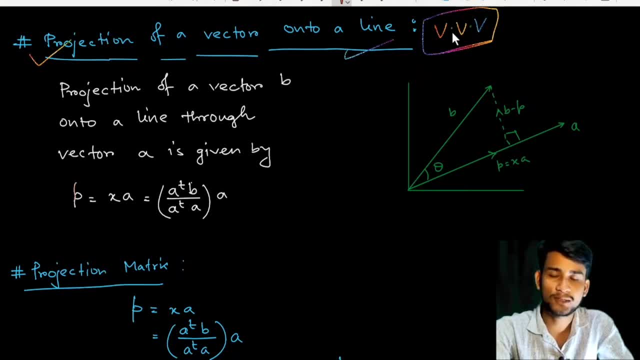 see the 5 year question paper, or 2 or 3 or 8 question paper. then a question from this section is also already comes. okay, it comes obviously okay. So projection of a vector b onto a line through vector a is given by p equal to x, a equal to a. 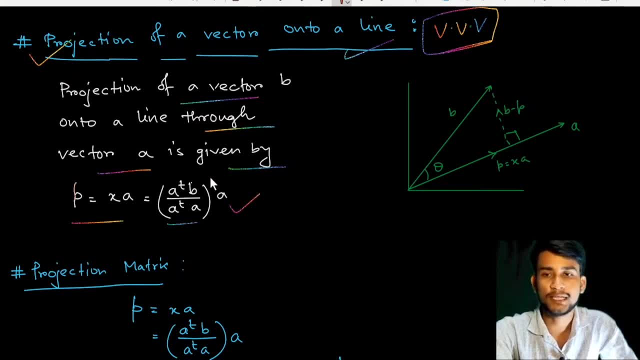 A transpose b by a transpose a into a vector. okay, this a and b are also vector. this is the image you can say: So this is the x axis and this is the y axis. this is the y axis or x- y plane you. 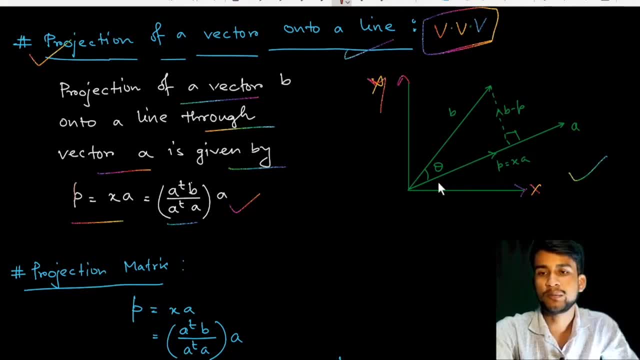 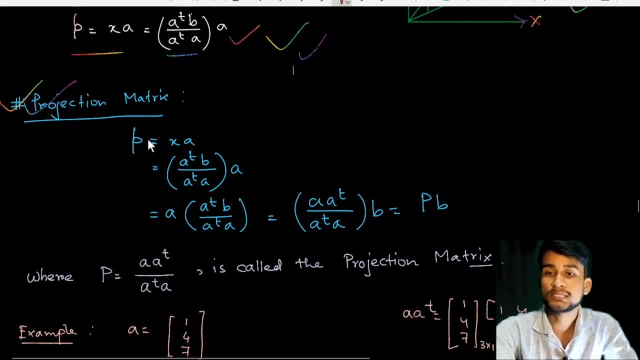 can say: onto a line. okay. So projection of a vector onto a line formula, is this okay? So here I take an example and projection matrix. you have to find the projection matrix, p equal to x, a equal to this. a transpose b by a. transpose a into a vector, this is equal to a. 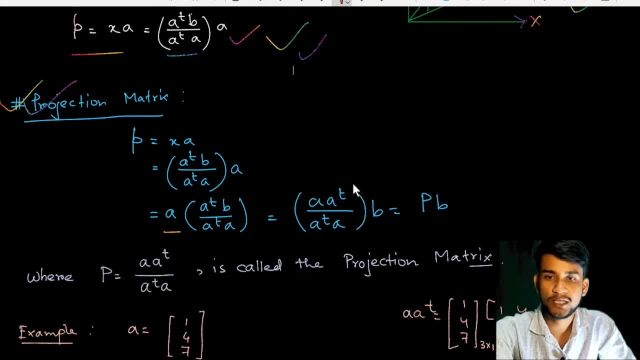 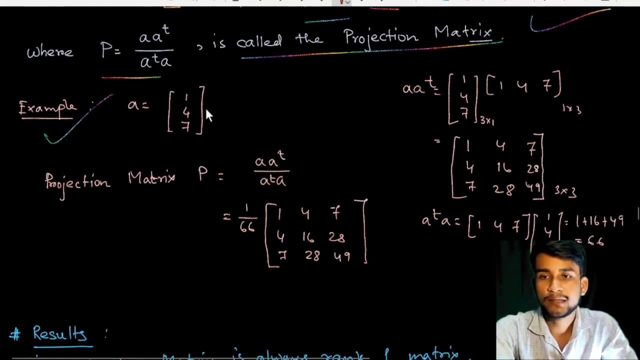 into a transpose b. A transpose a into b vector. this is equal to p vector and this p is equal to a. a transpose by a transpose a. this is called the projection matrix. okay, this is very important. just remind this formula. So let us take the example: a vector equal to 1, 4, 7, then we have to find the projection. 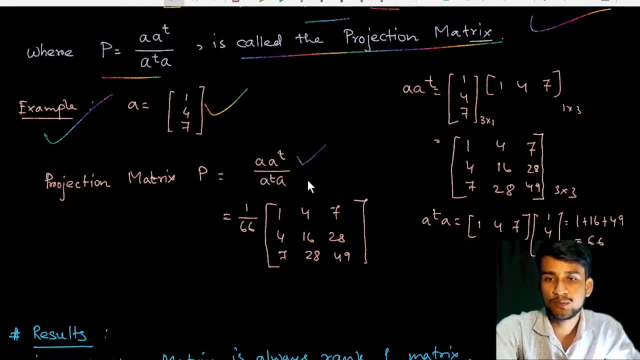 matrix, suppose. then the formula is a, a transpose by a transpose a. okay, So a, a transpose equal to this matrix and a transpose a equal to this matrix, and this is the simply 1 by 1, that is, and simple, any event. so this is equal to the matrix, this one, okay, so the projection matrix. 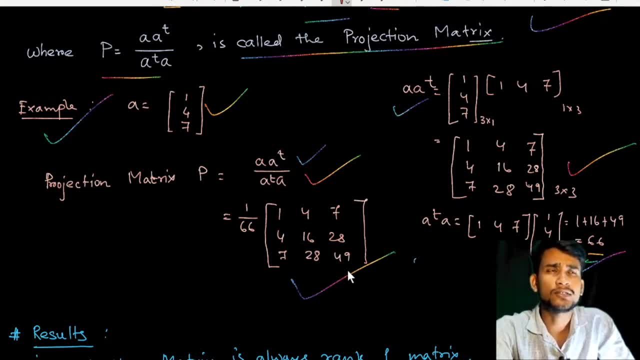 is this one, okay, and i think in a question paper- i think in which question paper there is a questions from this- you have to find the trace of the projection matrix, okay, so the question is very interesting questions. i think it is. it is a csr question or another question where i just 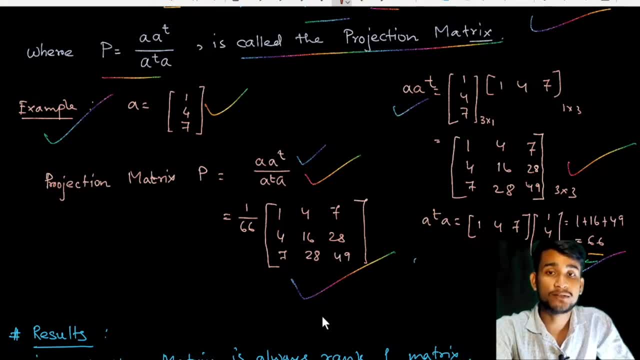 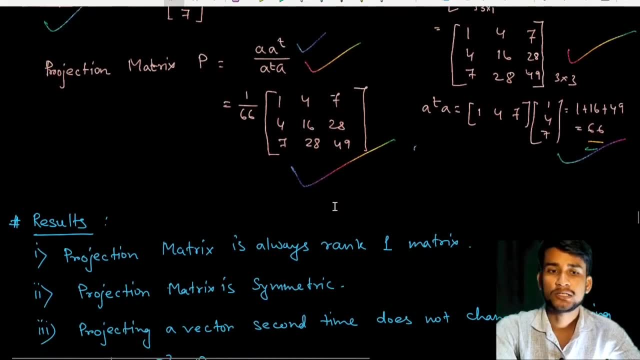 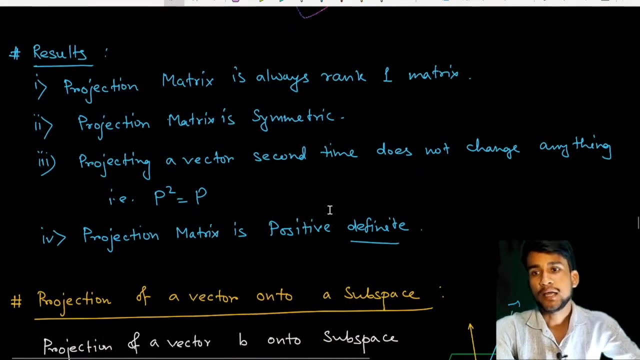 forget it. okay, so you have to find. the question was to find the trace of these matrix, i think. okay, so this is very important, so you can check and you can recall this and you can see this formula once before you going to the example. okay, and the result: then there is a projection. 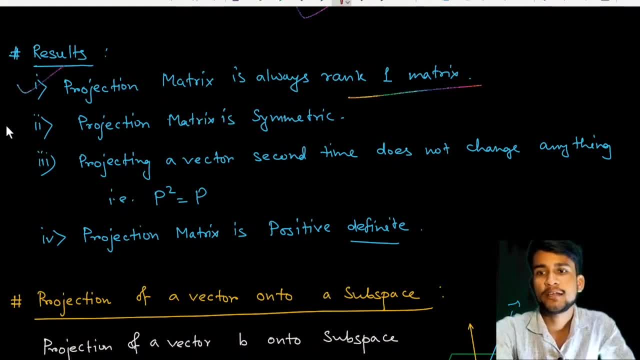 matrix on projection matrix. projection matrix is always rank one matrix. projection matrix is a symmetric matrix. projecting of a vector on a second time: do not change anything. that is p square equation equal to p: okay. projection matrix is a positive definite matrix- okay. so these two results are. 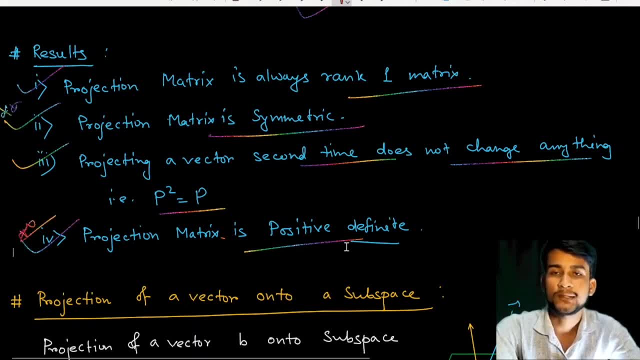 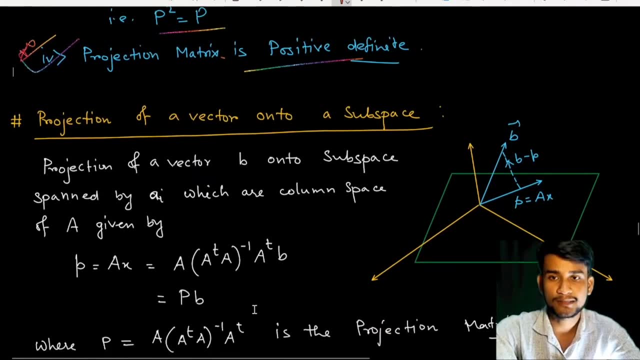 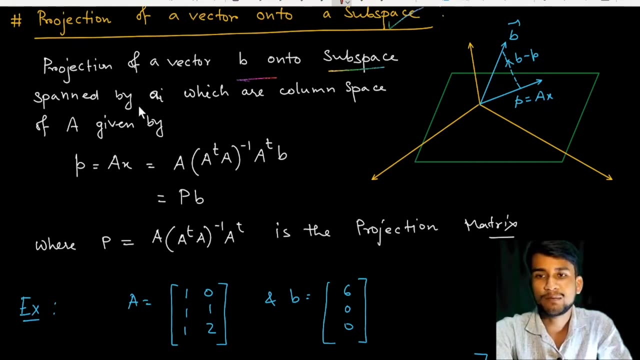 very important: symmetric and positive definite. okay, based on these two concepts or based on these results, the questions comes and says, and i just take the examples below: okay, so projection of a vector onto a subspace. okay so projection of a vector b onto a subspace spanned by a? i. 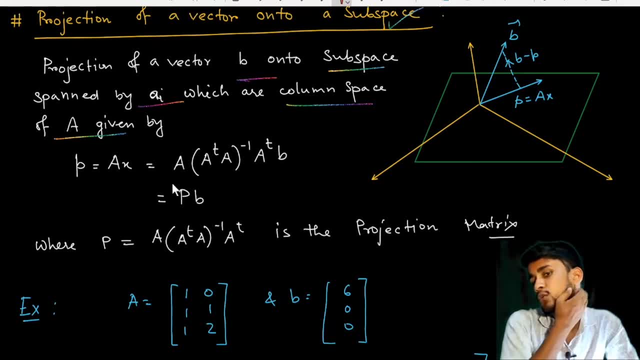 which are the column space of a matrix: a. p equal to a x. this is equal to a. a transpose a inverse a x. this is equal to a x. this is equal to a. a transpose a inverse a x. this is equal to a. a transpose b and this is equal to p b. okay, so p equal to this one. a. a transpose a inverse a. 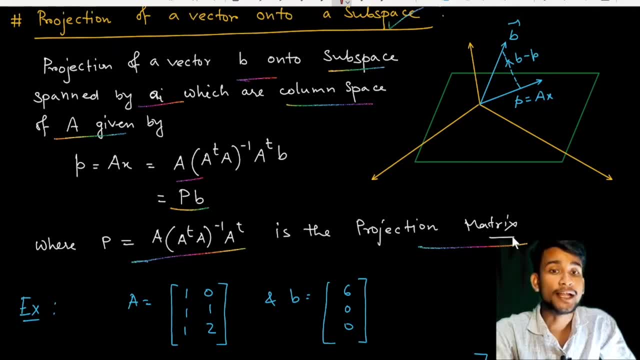 transpose is the projection matrix. okay, and here one thing is noted: that this matrix, this matrix a, is not necessarily a square matrix. okay, this may be a word, this may be a rectangular matrix, and most of the cases this is a rectangular matrix. this is a rectangle matrix. okay, so for that case, 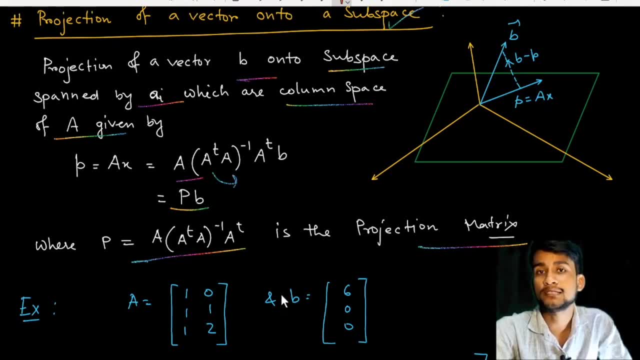 we don't, uh, have the determinant of the matrix, don't have the determinant of the matrix. that's why we can't change this one. that means we all know that a, b transpose, a, b whole trans, inverse. this is means what we write: b inverse, a inverse. but here we can't write it okay, because this is. 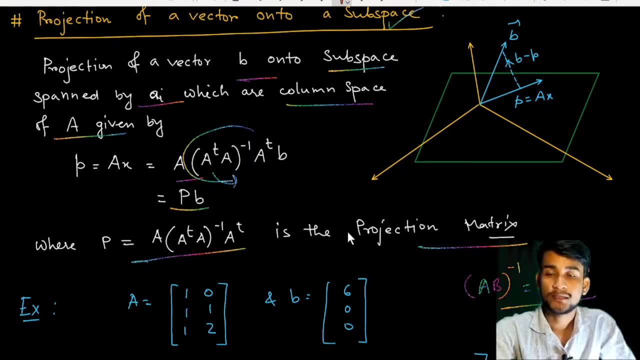 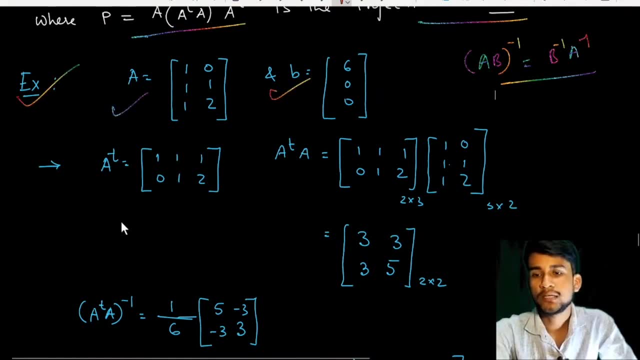 not a square matrix. okay, this is an important note. okay, so let us take an example: a equal to this, b equal to this. okay, so we have a square matrix. okay, so we have a square matrix. okay, so we have to find the projection matrix. suppose a, a transpose, a inverse, a transpose, okay, so a. 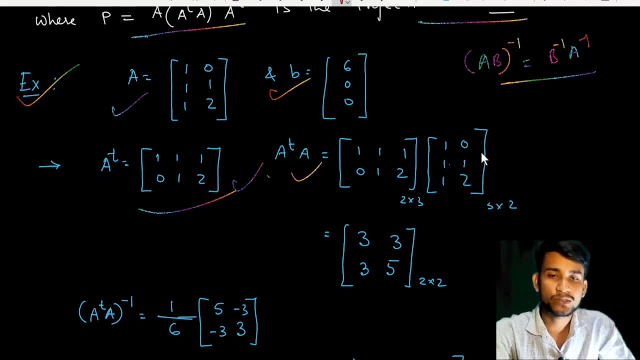 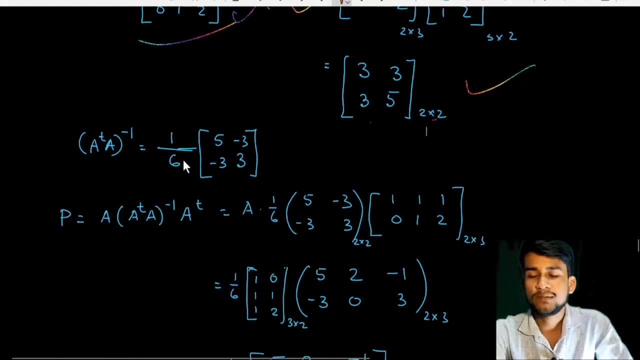 transpose equal to the a this one, a a transpose a equal to this one. so this is a 2 by 2 matrix 3, 3, 3, 5. okay, just you can check it. okay, so a transpose a inverse, this is equal to this one is the simple. 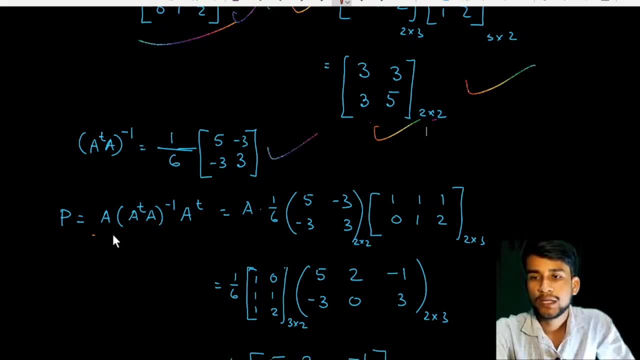 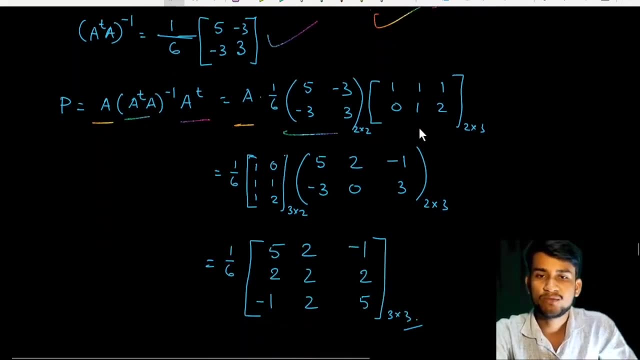 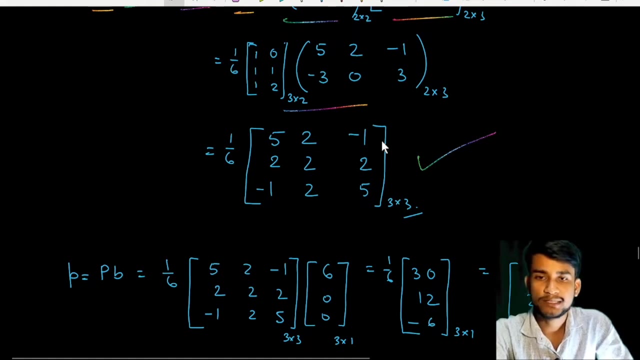 inverse, 1 by 6 into this one and p equal to. therefore, a, a transpose, a inverse, a transpose. okay, so that means what that means this: a, a transpose, a inverse into a transpose. okay, so this is a simple matrix multipliers and we, and we get finally what get finally, 1 by 6 into this is the. 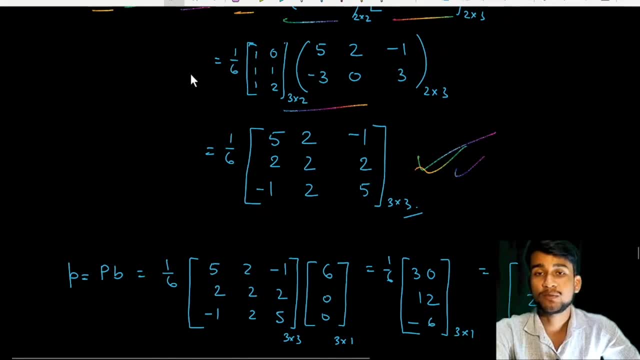 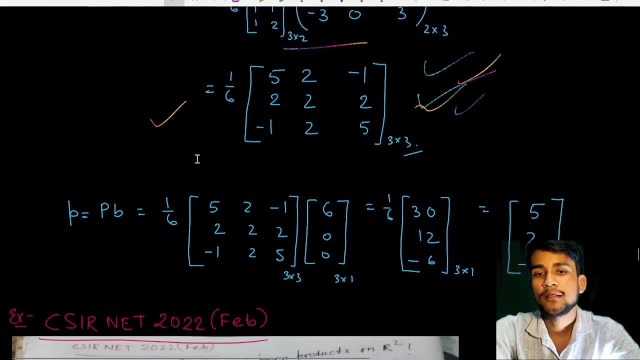 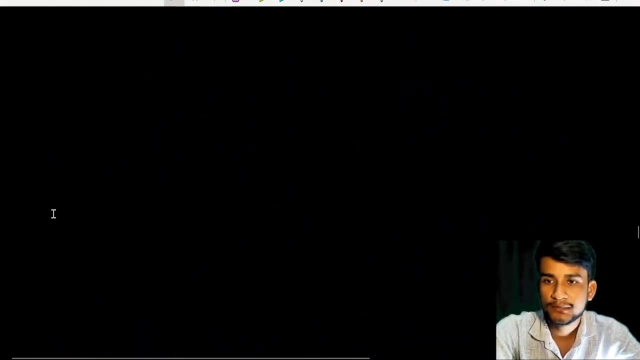 matrix. okay, so p matrix, that is projection matrix for a vector, a projection of a vector to a subspace. okay, this is the projection matrix. okay, and the formula you have find it okay. so p equal to what the projection matrix and the p is just here you can check small p. this is equal to capital p. this 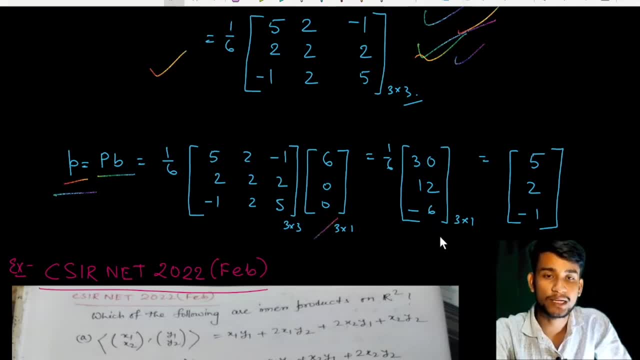 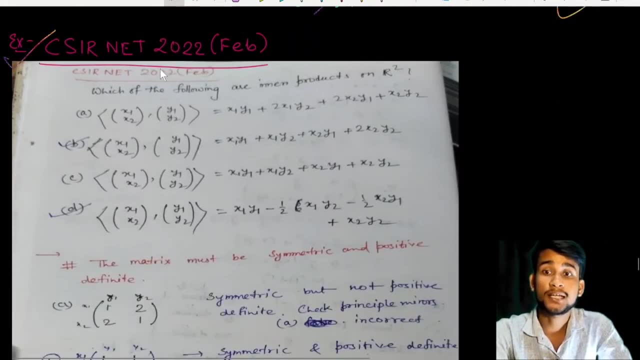 matrix into b vector and b vector is suppose, if we take this one is a b vector, then this is the small p matrix matrix. okay, now let us take the example, and this is the current question, from cs and net 2022. okay, the question says that which of the following are inner products based on r2? 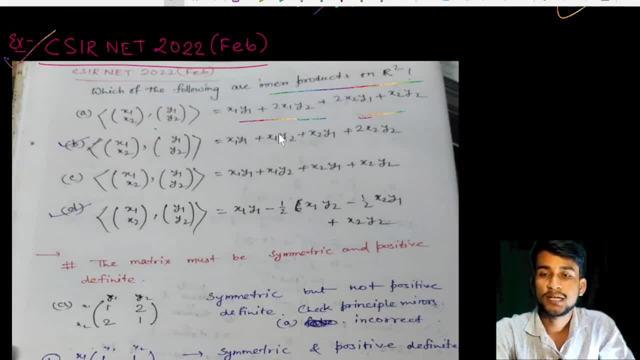 okay, so these are the given. okay, so this is the given. this is a very easy question which comes in cs and net 2022. okay, the two result is needed to solve these questions. okay, one is what: the projection matrix or the inner product space? the matrix is um symmetric and positive. 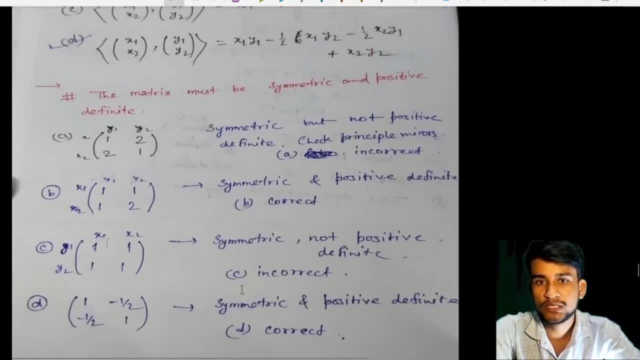 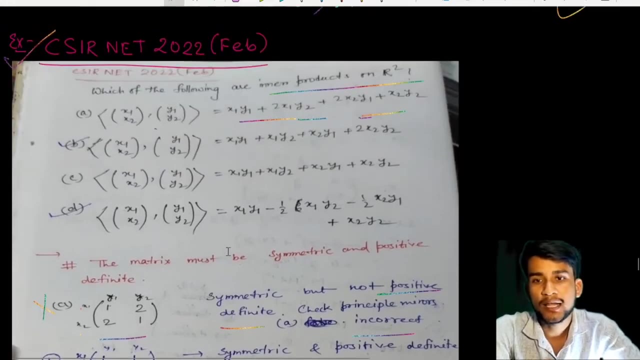 definite. okay, so we just write the matrix corresponding to the given inner product. okay, so x1, x1, x2, y1, y2. this matrix is symmetric but not positive definite. therefore, this is incorrect one. just we have to check and up to this. according to this, we just write the matrix and check what. 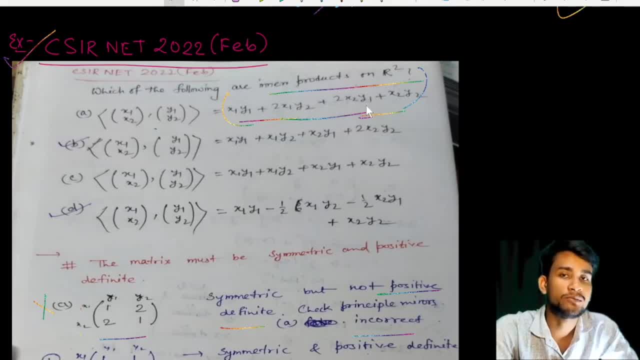 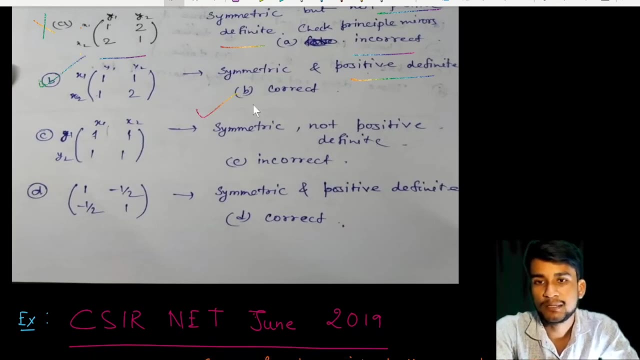 the matrix is symmetric and positive, definite or not. if one of these fails, then we say that this is not an inner product. okay, so we just take it. check those inner product. so this is symmetric and positive. definite, be correct option and see the matrix: this one symmetric and positive. 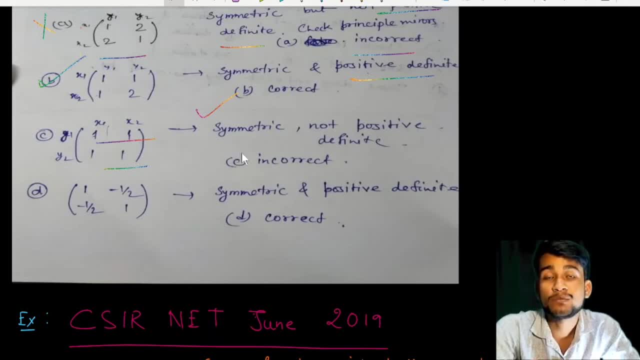 definite and to check positive, you need you just check the principal minors, okay, you all know that i think the principal minor method to check, uh, the positive or not. so this is symmetric and positive definitely, okay, so see symmetric matrix. clearly this is a symmetric matrix and positive definite mix, one by one, principal minor and this 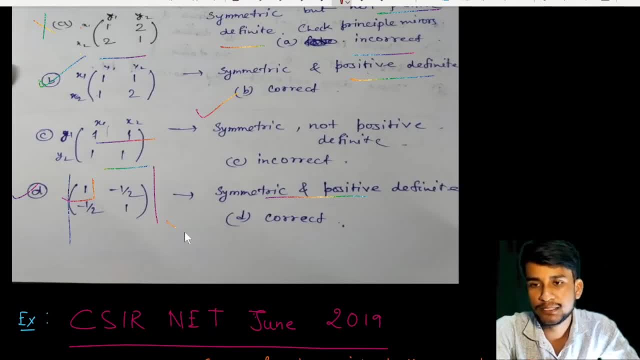 one and two by two. principal minor means the data of the this. this is greater than zero or not. okay. so if the principal minus are greater than zero, that means the matrix is positive. definite matrix: okay, matrix. okay. so here b and d options are correct. okay, this is very simple question. you all. 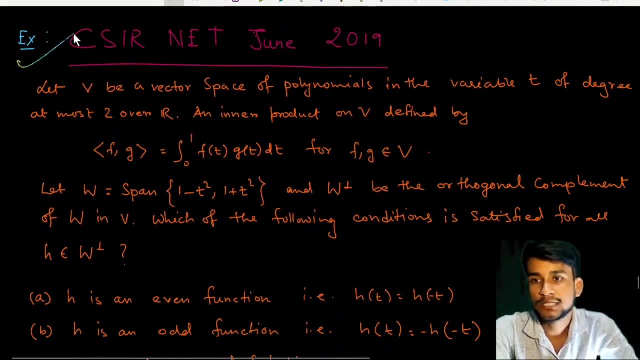 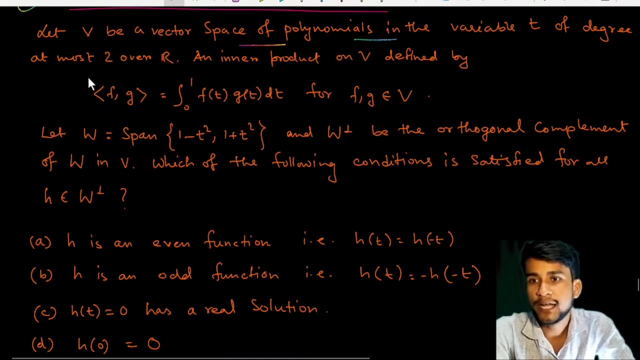 have to solve this question. okay, so there is a questions. csr net, 20 june, 29th instant. let v be a vector space of polynomials in the variable t- okay- of degree at most 2 over r and inner product b is defined by f and g. this: 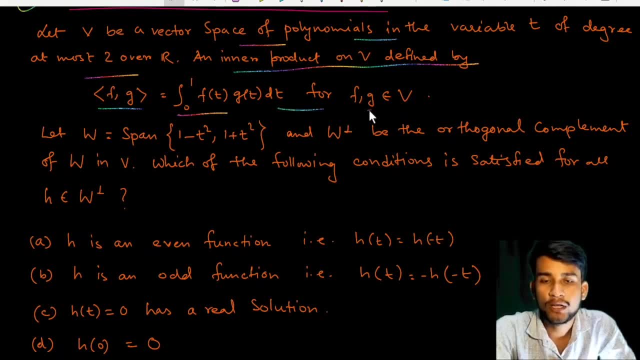 is equal to integration. 0 to 1 ft. gt, dd for f. g belongs to b. let w equal to span of this one and w perpendicular be the orthogonal complement of w in v, then which of the following condition satisfies, for h belongs to w, perpendicular. okay. 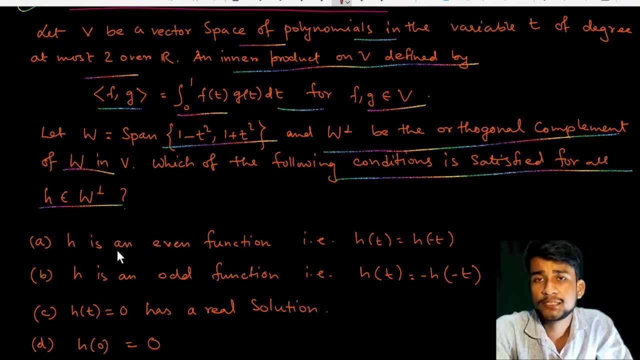 so here we have to- we- the question is based on the word- to characterize the function h. okay, so we have to first find, or we have to try to find, the function h and then we can say whether it is even function, whether it is odd function and it is a real root or not, okay, and whether it is zero or 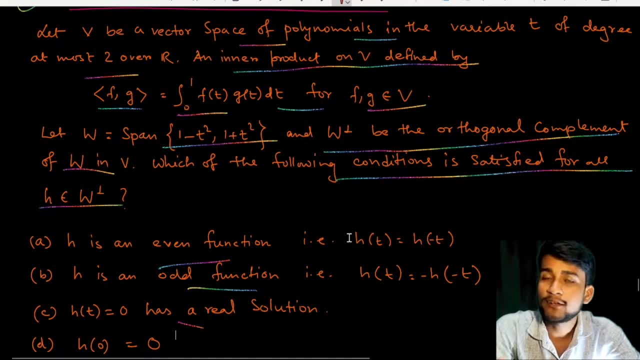 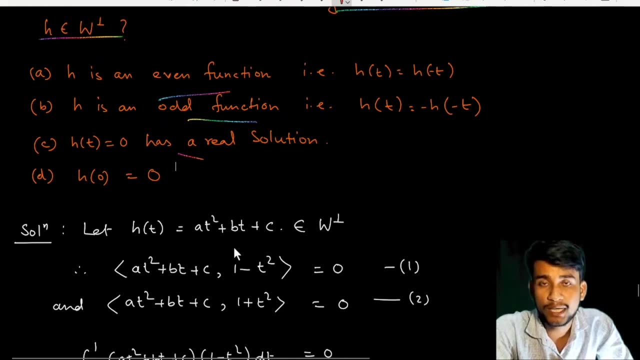 not okay, so we have to just uh try to find the function h. okay, so a let us take, since, uh, the functions or the polynomials are at most two degrees. therefore we take a zero, so we have to general polynomial of degree 2.. So h t equal to this one, we take the general polynomial. 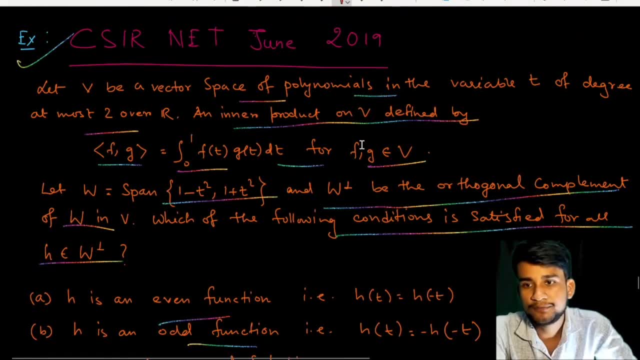 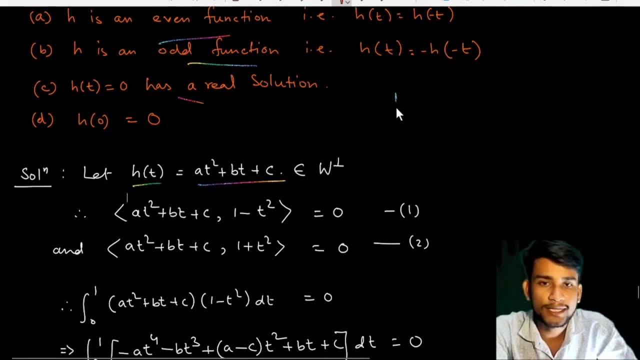 Now it says that what w equal to span of this one and w belongs to h perpendicular, That means the h, that means what h and these two vectors, f and g, are what orthogonal complement to each other or orthogonal set of vectors, And so that means these two inner product goes to 0 and 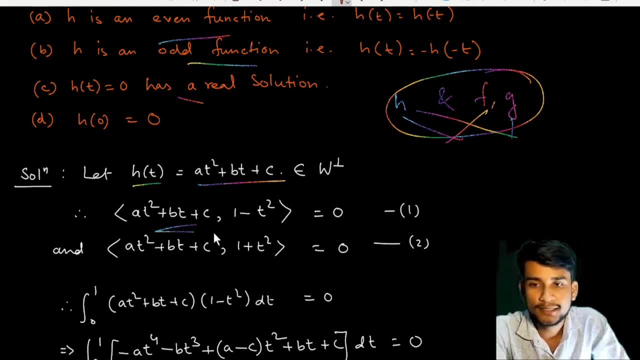 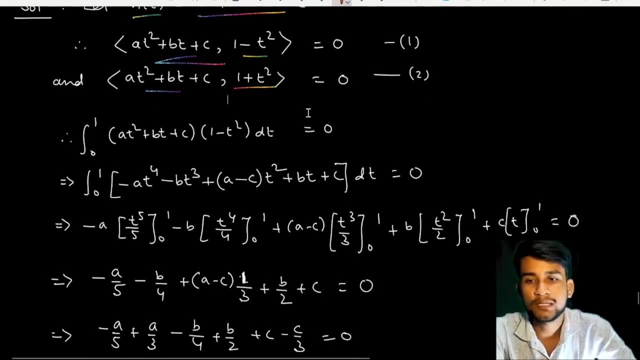 these two inner product goes to 0.. So we just write this: this is h and this and this: this inner product goes to 0. Therefore, we just apply the method given here and 0 to 1 into this one. 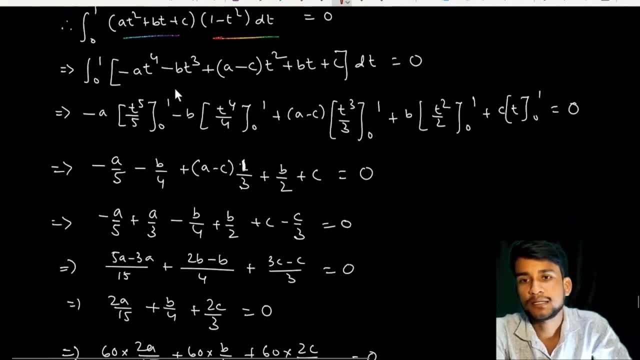 this one, this is equal to 0, just simple integration. So we, just simple integration, calculate this one and we get a relation in this: So 2 a by 15 plus b by 4, plus 2 c by 3,. 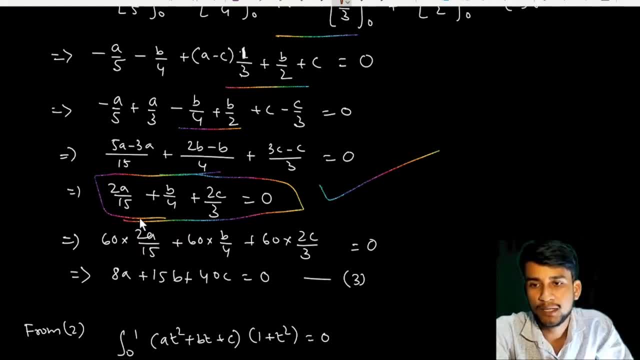 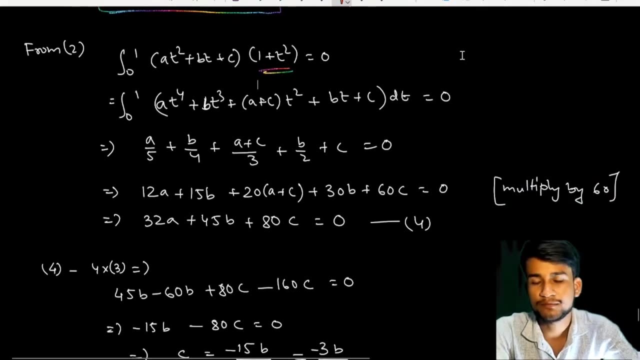 this is equal to 0.. So if we just multiply by the LCM of these three, then we get 80 plus 15 b plus 14 c. this is equal to 0.. And similar process for taking this one, But by taking this second vector we just get. 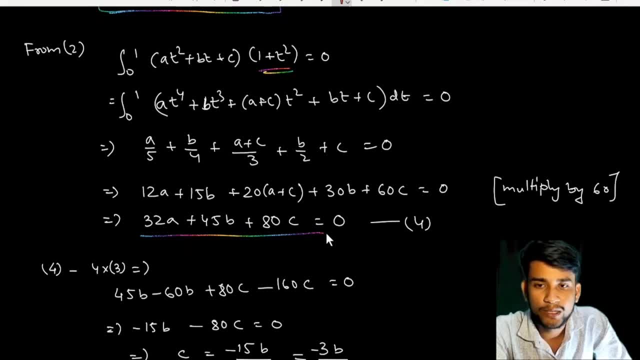 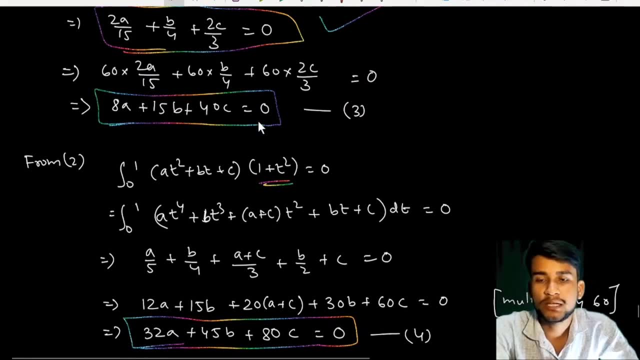 this one: 32 a plus 45 b plus 18 c, this is equal to 0, multiply by 60. Therefore, 4 minus. we just have to calculate. there is two equation and three unknown. Therefore, we cannot solve the system in general, So we have to choose any one. 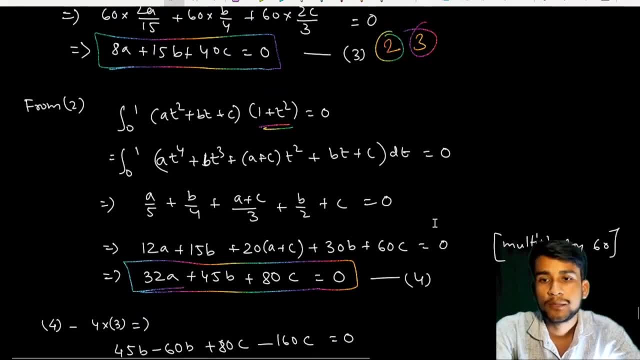 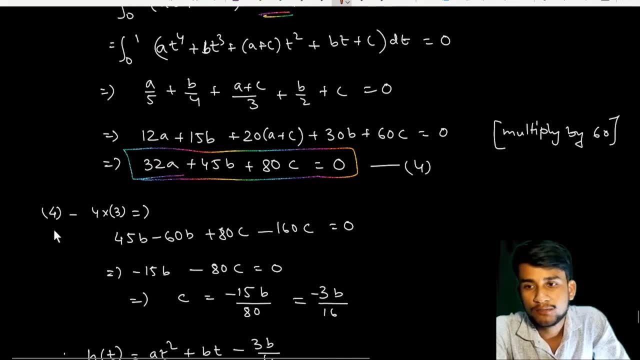 of the constant. So if we first eliminate any one of these two, three constant, then we get or parameter, we get 40, 4 minus 4 into 3, this gives we eliminate a, So we get a relation. 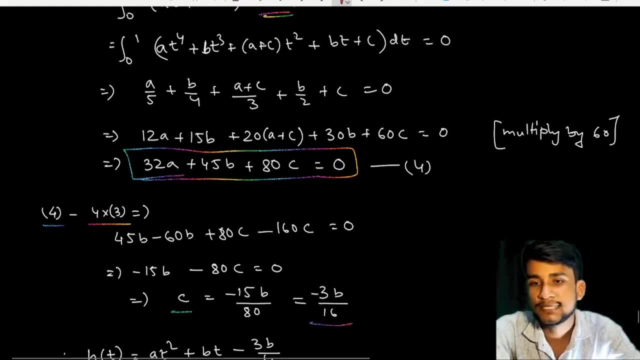 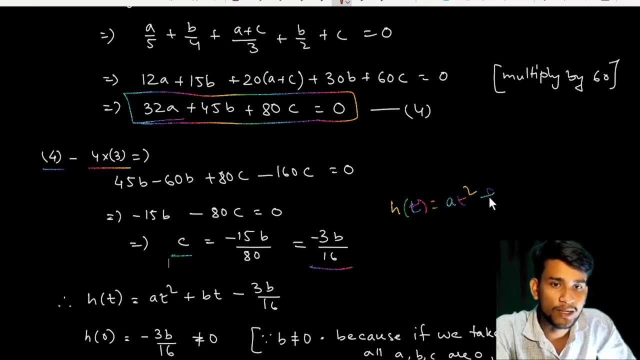 between c and b. Therefore c equal to minus 3 b by 16 a. Therefore we just write where, since h, t, this is equal to a, t square plus b, t plus c. Therefore we just eliminate one constant. So 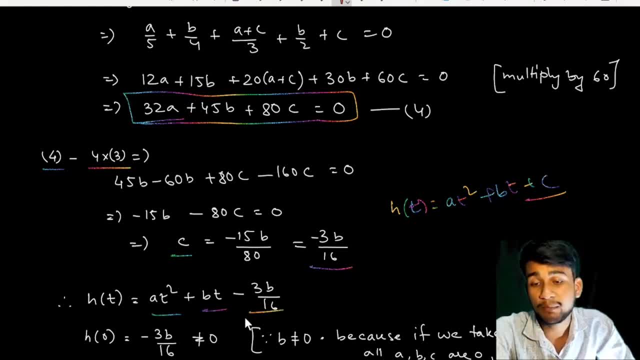 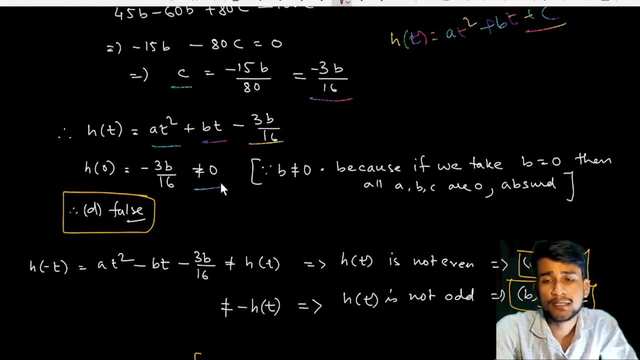 h? t equal to a t square plus b t plus 3 b by 16,, minus 3 b by 16. Now h 0 equal to 3 b by 16, which is not equal to 0. And it is 0 only when b equal to 0. But if we get b equal to 0,, 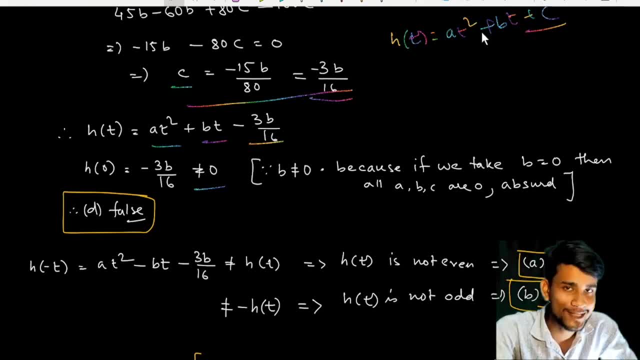 then from this relation, c is also 0, and c is also 0 means a is also 0. Therefore there is- this is an abstract, abstract situation- If a, b, c are all 3, 0, therefore there is nothing to do this problem. So this is: 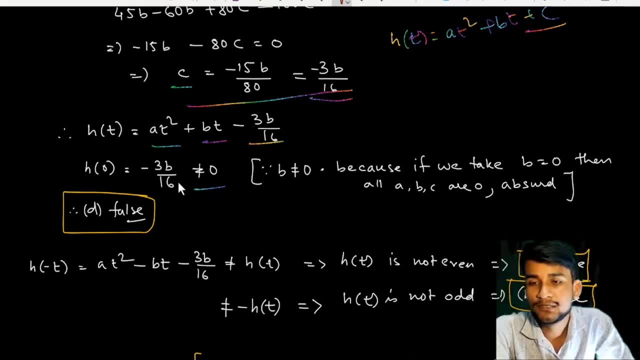 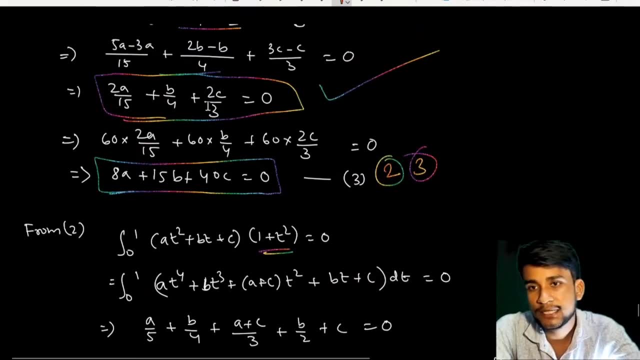 this is case is not true. That means the h 0, this is b- is not equal to 0. So d is false option. We clearly say that The d option is what d option is? I think h 0 equal to 0.. So d option. 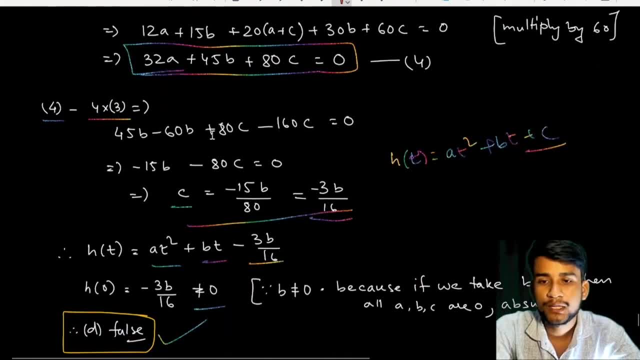 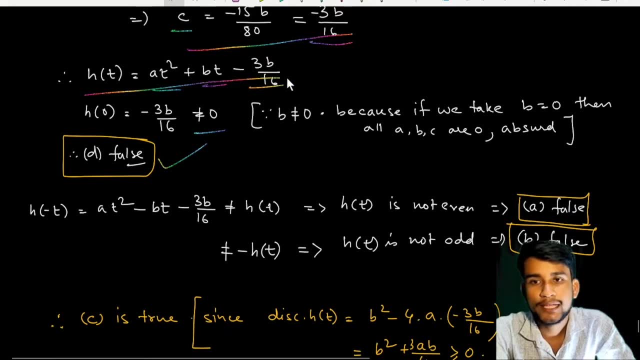 is false option. Now it comes to the another options. Now, h t equal to h t equal to. we just write this one. Therefore, h of minus t is not equal to h t and h of minus t is not equal to. 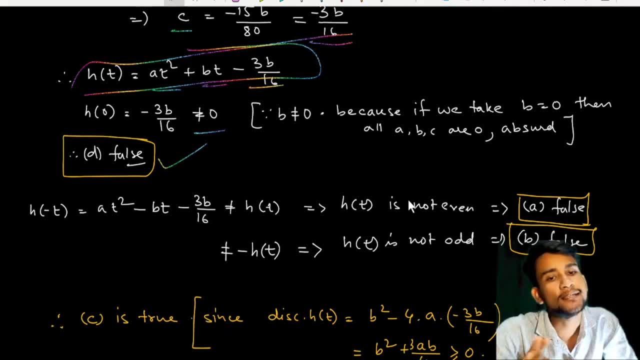 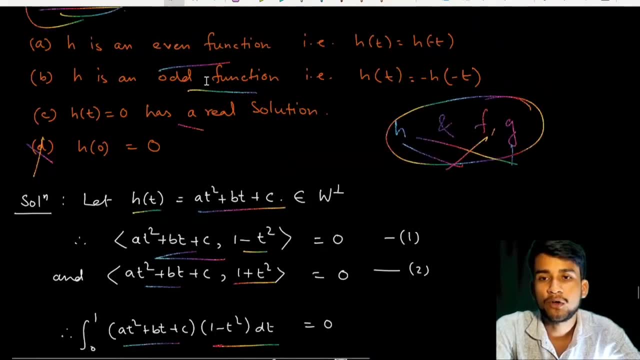 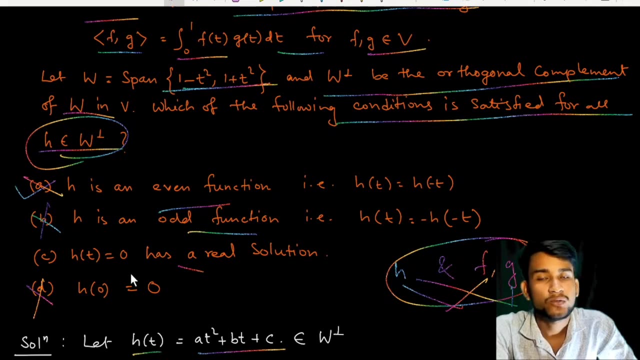 minus of h, of minus t. Therefore this is not a even function and this is not a odd function. Therefore a option is also false and b option is also false. Therefore, only options remaining is: a is false and b is also false. Therefore the remaining option c, we can say obviously: 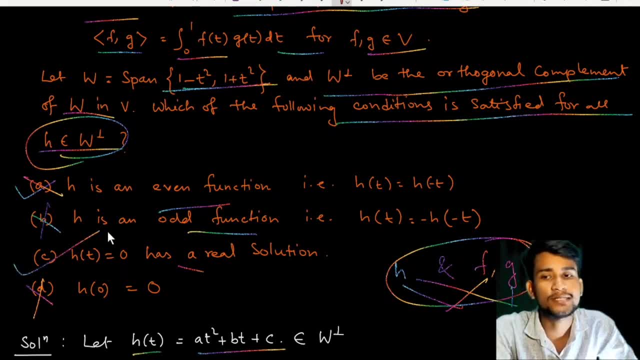 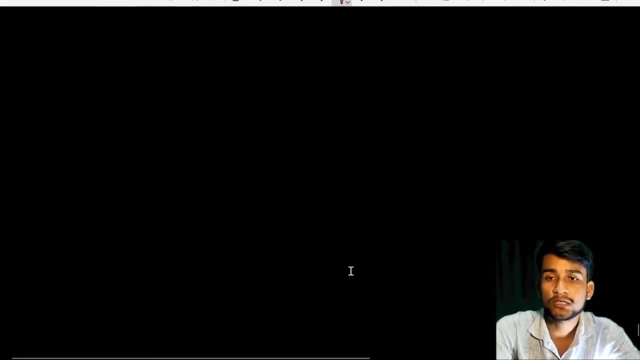 if we discard the remaining 3 options, therefore, we can say it obviously that the third option- h equal to 0, has a real solution. So this is true option. Also, we can check just a minute. 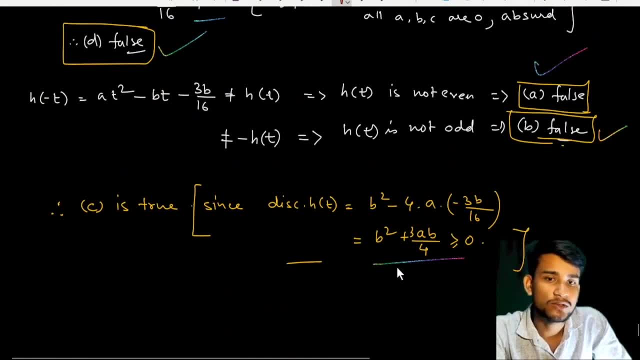 Also, we can check the discriminant. this one, this one is greater than 0. Therefore, the greater equal to 0, we can say, therefore, we can say that the h? t function has a real solution. So we do not need to check out. if we discard 3 options, then we can obviously say that the 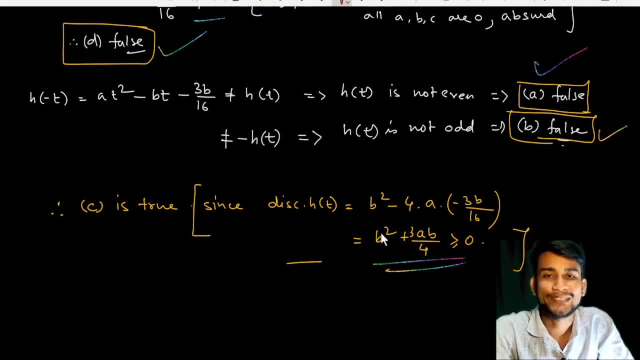 remaining option is true if the question is right. So this is the content and this is a to the point discussion on inner product space. I think this video helps you a little bit, or helps you something to your for your preparation. So if you like the content, 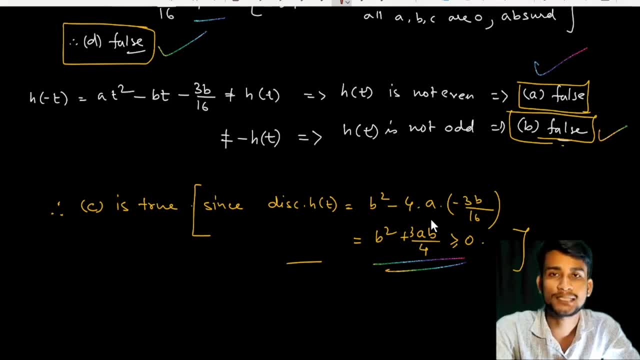 then please give a like to the video, share with your friends and subscribe to the channel. Thank you, friends. See you again in the next video.